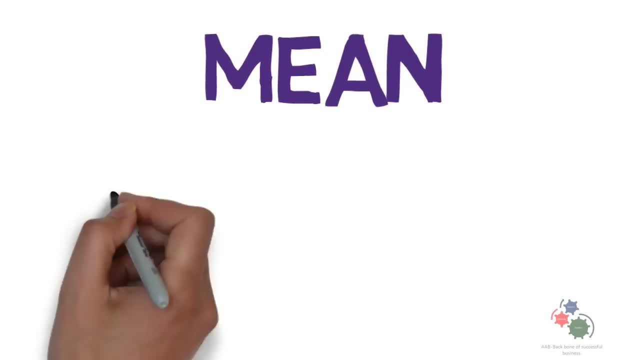 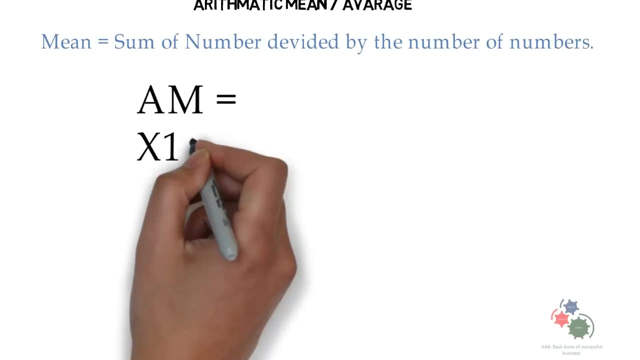 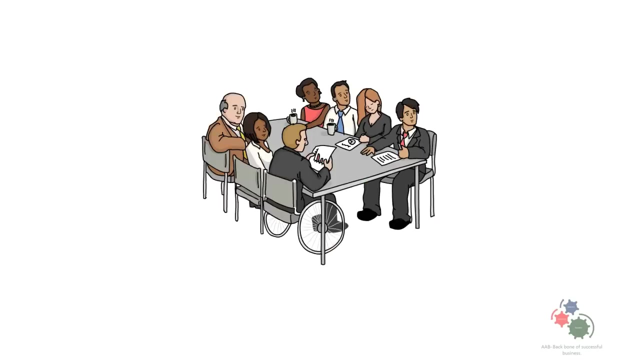 VIF Mean, We can say Arithmetic Mean, or Average Sum of numbers Divided by number of numbers: A-M, x1 plus x2 plus x3, dot, dot, dot, xn divided by n. These are the salary of group of people. If you want to know what is the mean salary of these, 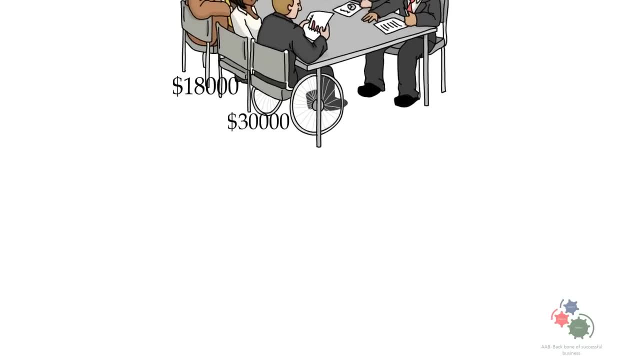 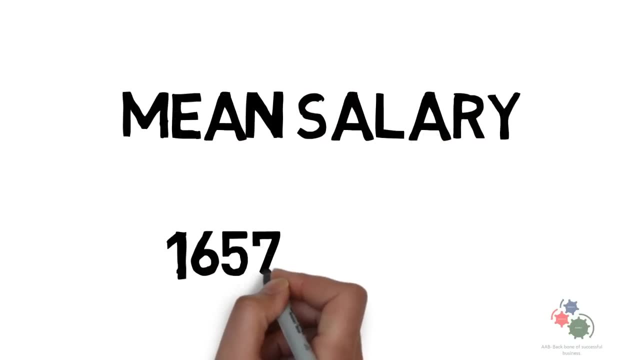 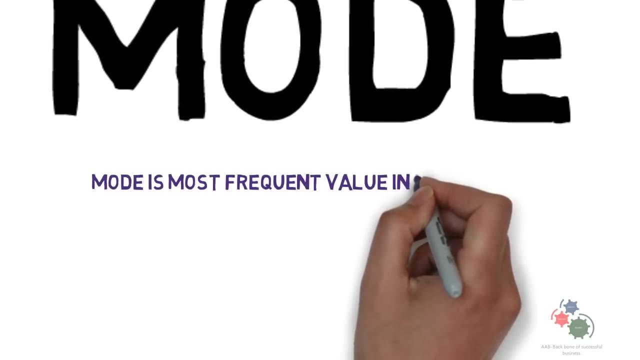 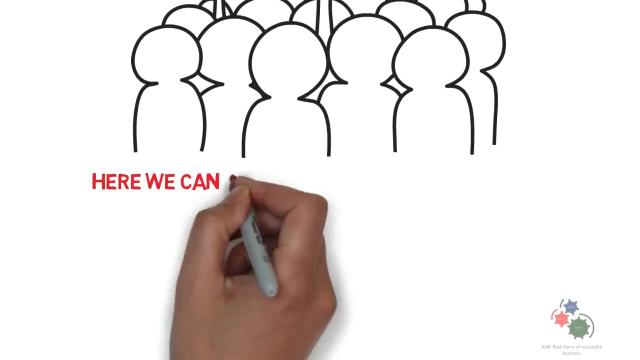 people. Mean salary is equal to sum of all salaries divided by number of people, Here 16571.42.. Mode Mode is most frequent value in the data set. Here most of the people's age is 30. And we can say mode age of the group is 30.. 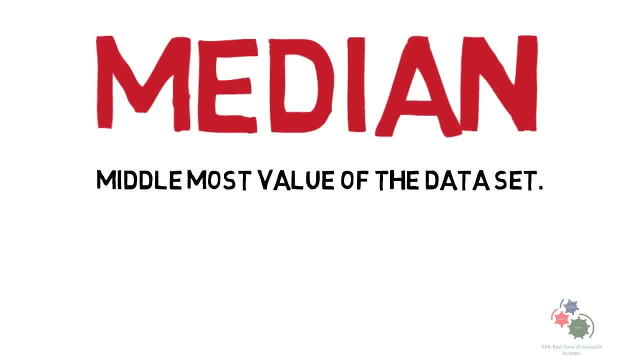 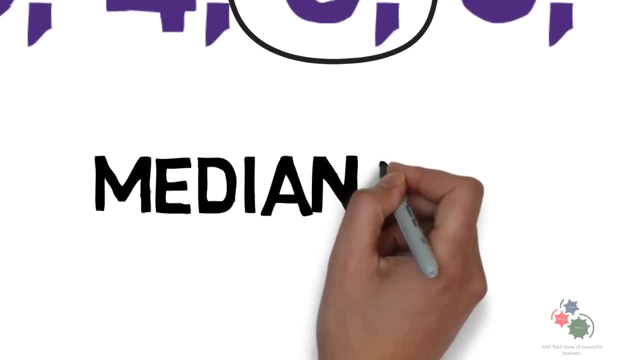 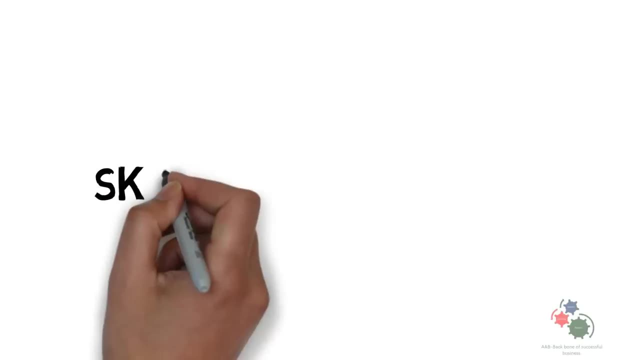 Median – Middle most value of the dataset. Here set of data between 1 to 9.. Here median is 5.. The median is the value separating the highest half of the dataset from the lower half. Skewed and kurtosis. To understand skewed and kurtosis we need 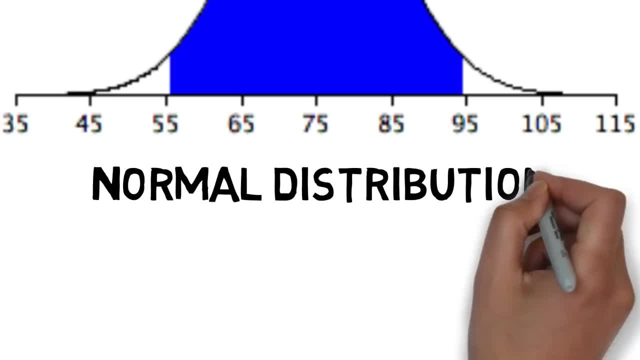 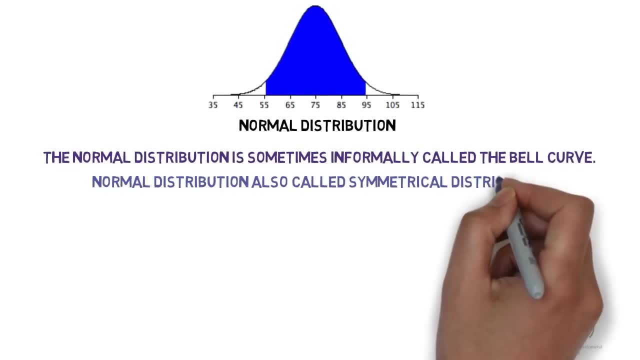 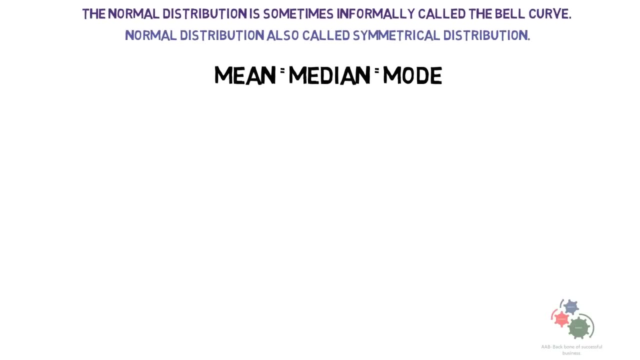 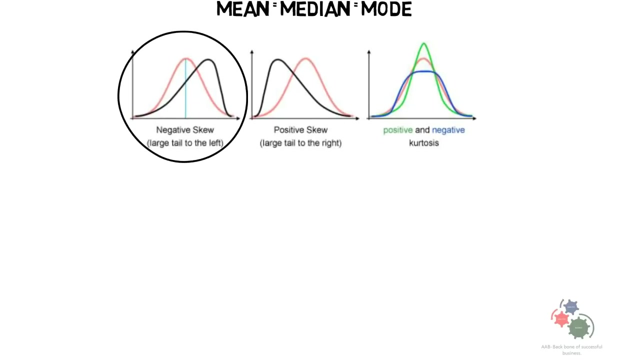 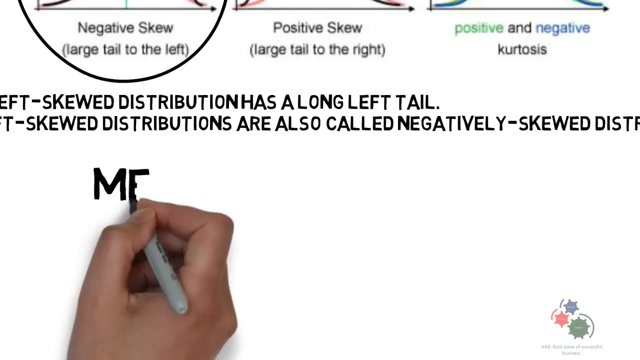 to understand normal distribution first. The normal distribution is something informally called as weld curve. The normal distribution, also called symmetric distribution, where mean is equal to median, is equal to mode Left skewed distribution. A left skewed distribution has a longer left tail. Left skewed distribution are also called negative distribution, where mean lesser than median. 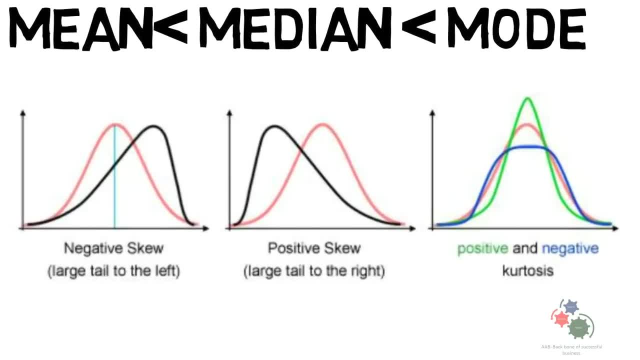 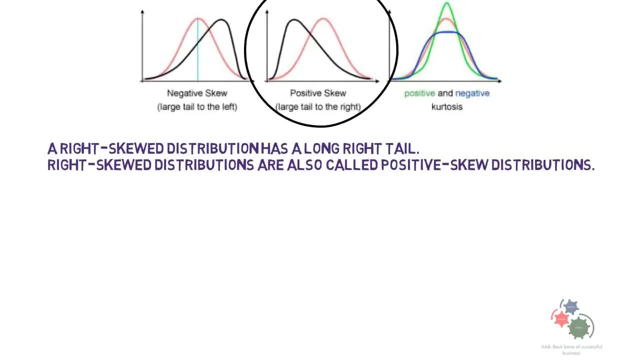 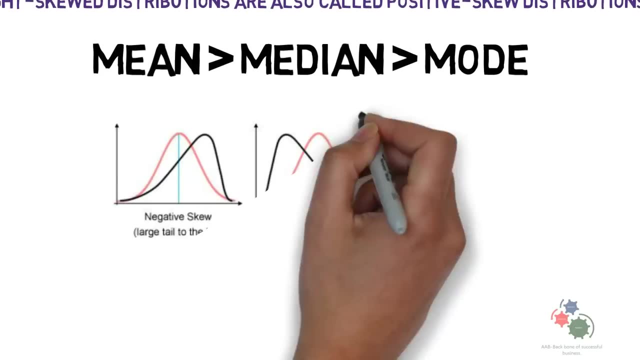 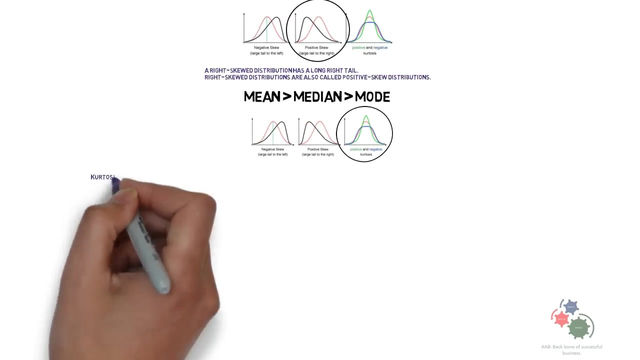 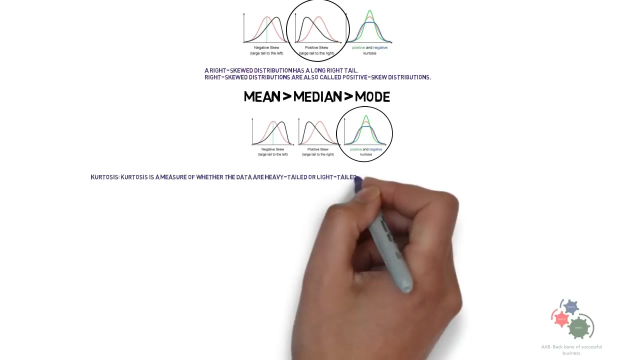 lesser than mode. Right skewed distribution. A right skewed distribution has a longer right tail. Right skewed distribution are also called positive skewed distribution, where mean is greater than median is greater than mode Kurtosis. Kurtosis is a measure of whether the data are heavily tailed or light tailed related to a normal distribution. 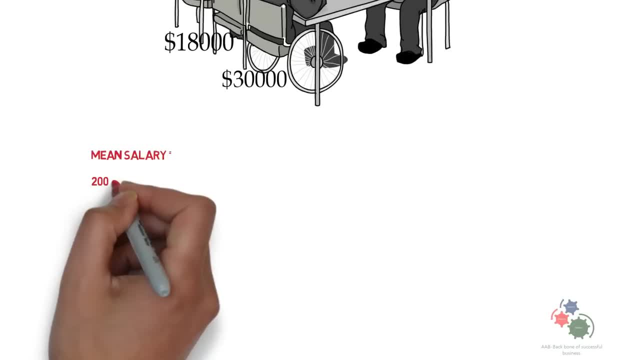 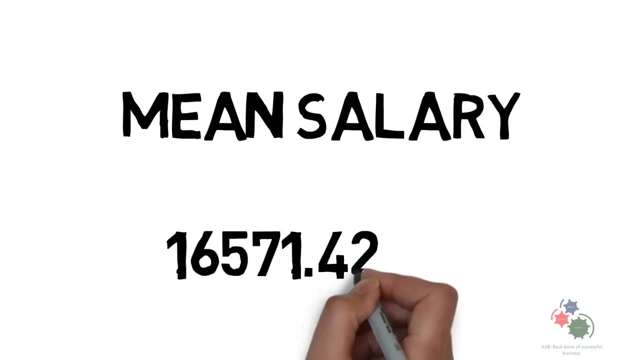 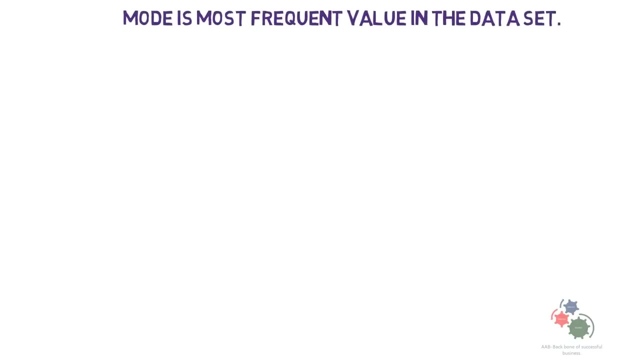 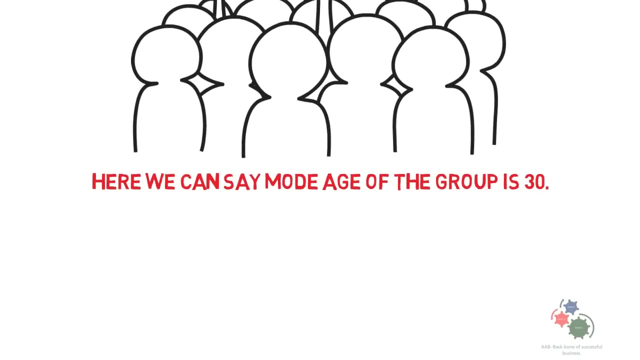 Mean salary is equal to sum of all salaries divided by number of people, Here 16571.42.. Mode Mode is most frequent value in the data set. Here most of the people's age is 30.. Here we can say mode age of the group is 30.. 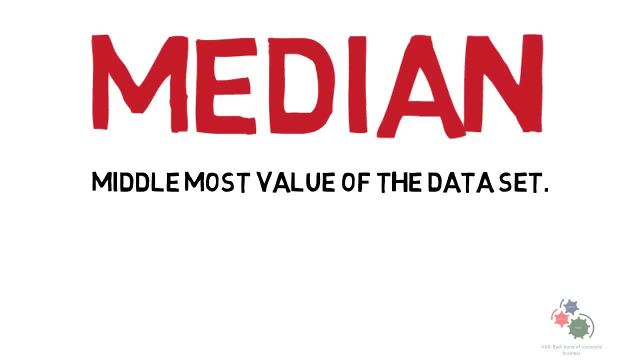 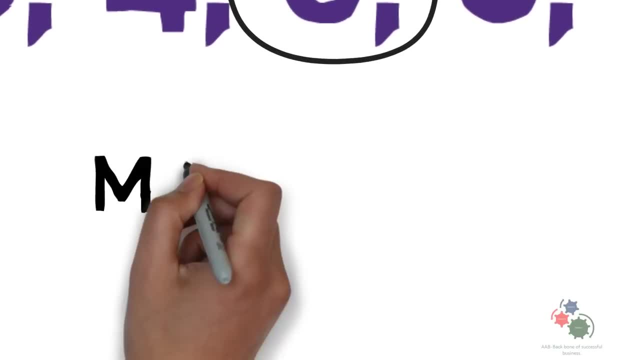 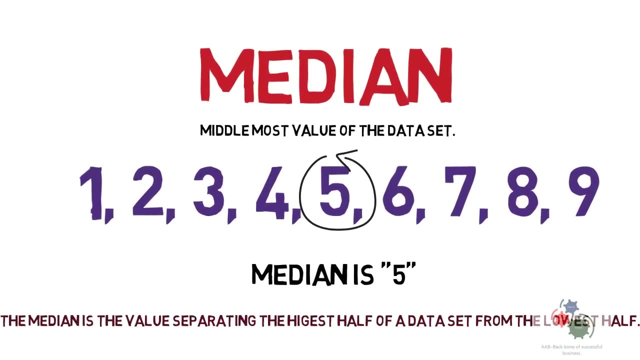 Median Middle: most value of the data set. Here set of data between 1 to 9.. Here median is 5.. The median is the value separated by 1.. Here median is 5.. The median is the value separating the highest half of the data set from the lower half. 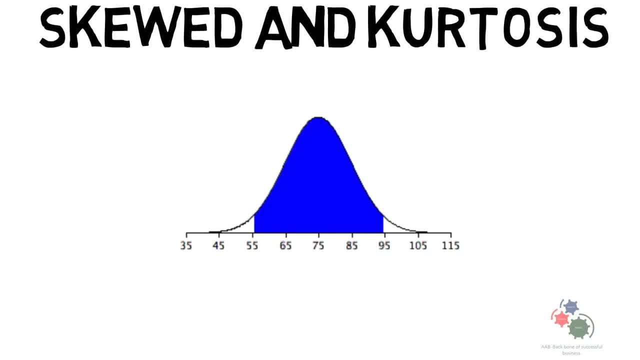 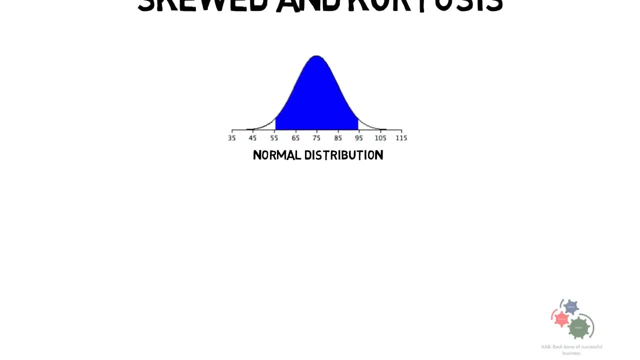 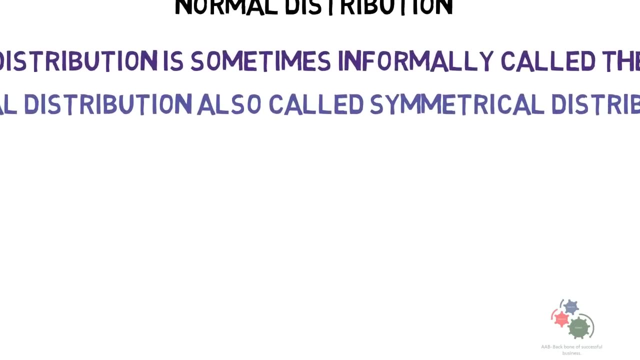 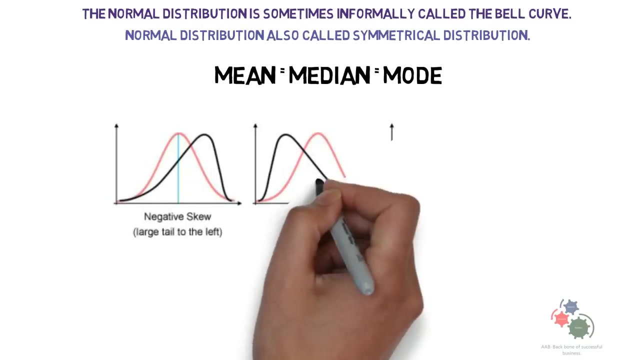 Skewed and kurtosis. To understand skewed and kurtosis, we need to understand normal distribution first. The normal distribution is something informally called as Weld curve. The normal distribution, also called symmetric distribution, Where Median is equal to median is equal to mode. 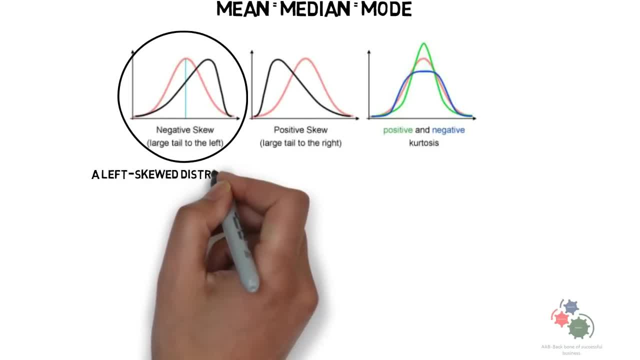 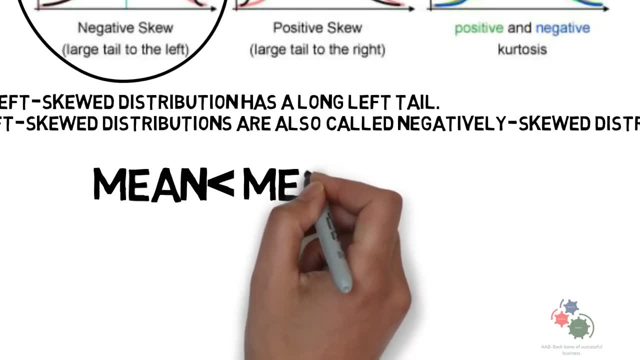 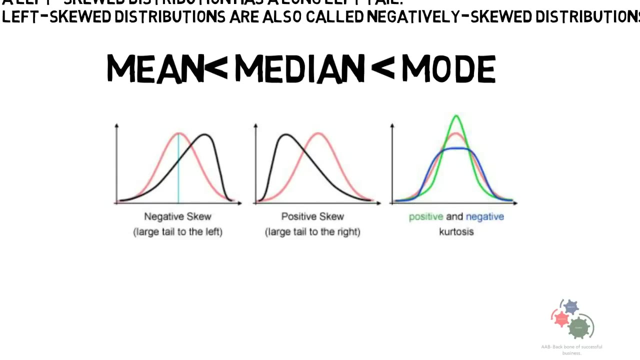 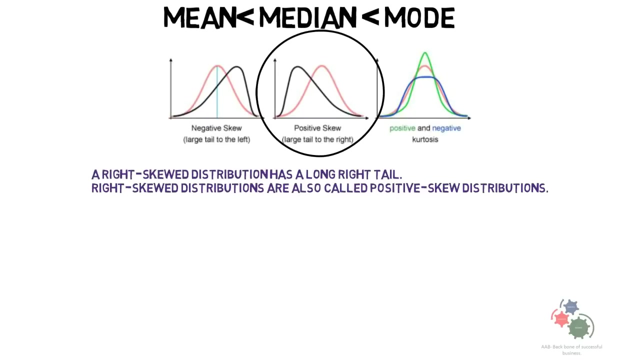 Left skewed distribution. A left skewed distribution has a longer left tail. Left skewed distribution are also called negative distribution, Where Mean lesser than median, lesser than mode. Right skewed distribution Has a longer right tail. Right skewed distribution are also called positive skewed distribution. 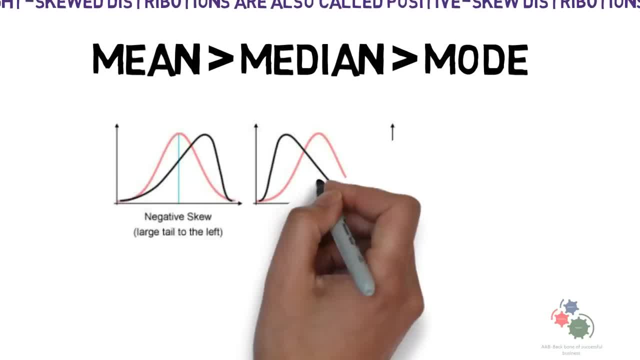 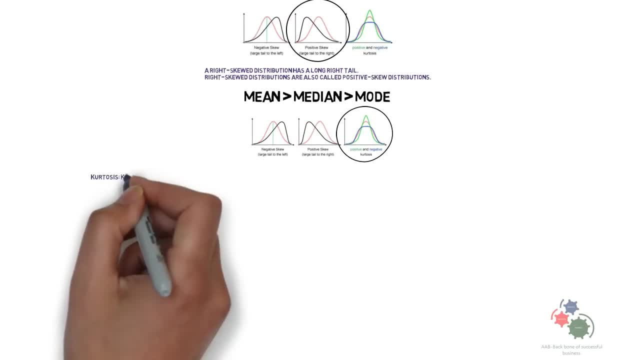 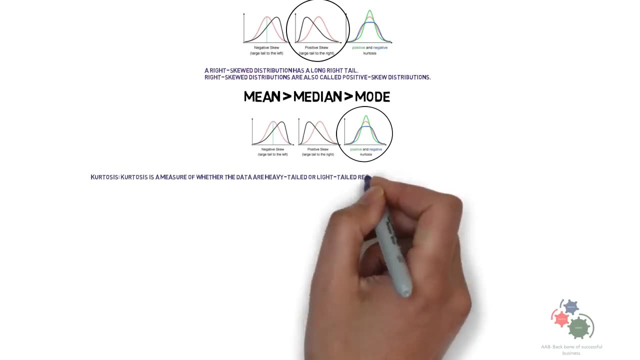 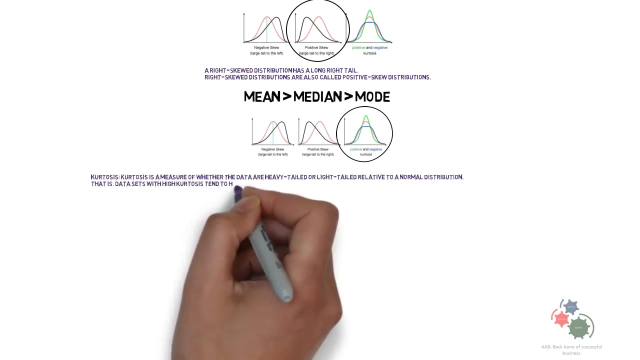 Where Mean is greater than median is greater than mode Kurtosis. Kurtosis is a measure of whether the data are heavily tailed or light tail related to a normal distribution, That is, Data which high kurtosis tends to have heavily tails or outliers. 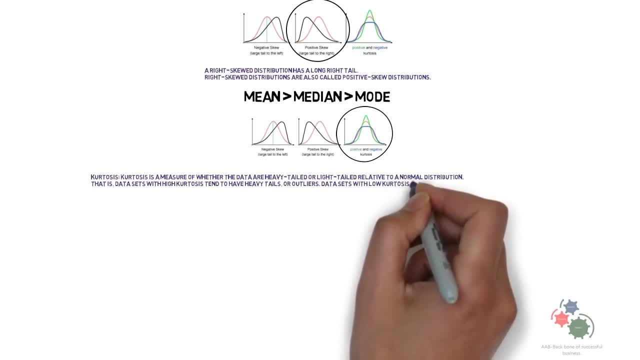 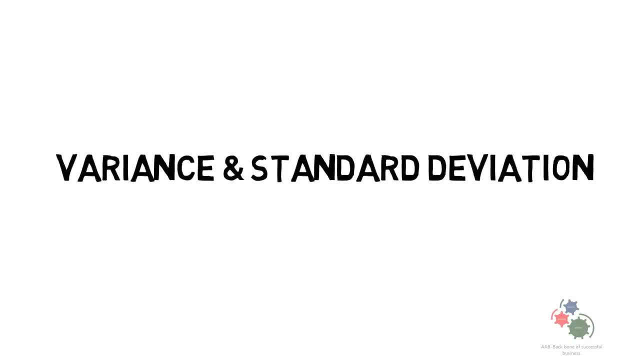 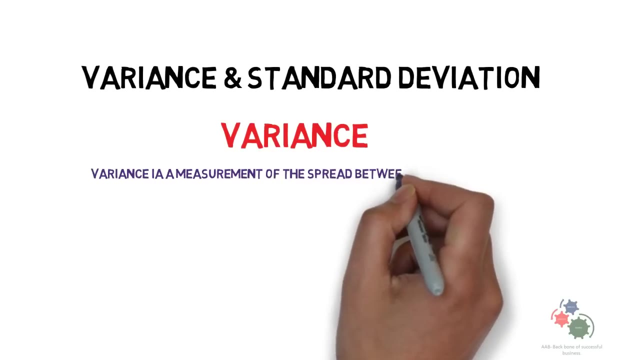 Data with lower kurtosis tends to have light tails or lack of outliers. Variance and standard deviation Variance. Variance is measurement of the spread between numbers in a data set. The variance measures how far each number in the data set is from the measurement of. 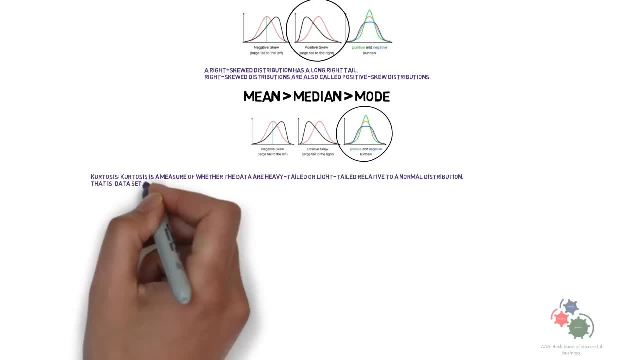 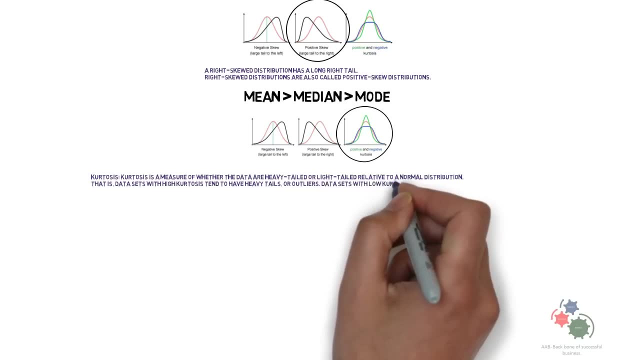 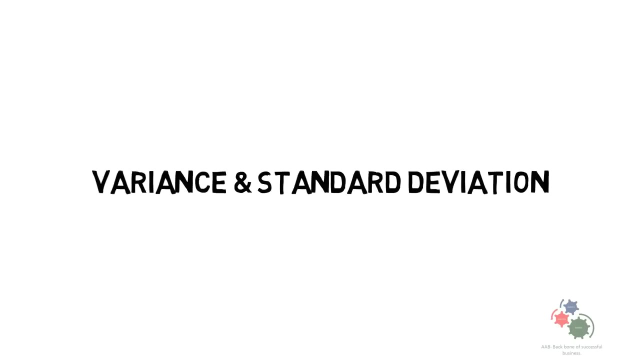 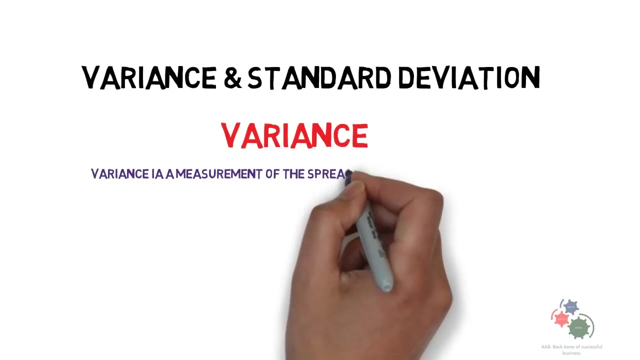 That is data which high kurtosis tends to have heavily tailed or outliers. Data with lower kurtosis tends to have light tails or lack of outliers. Variance and Standard Deviation Variance is measurement of the spread between numbers in a dataset. 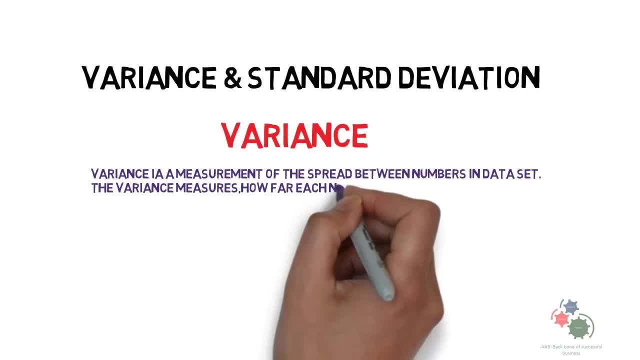 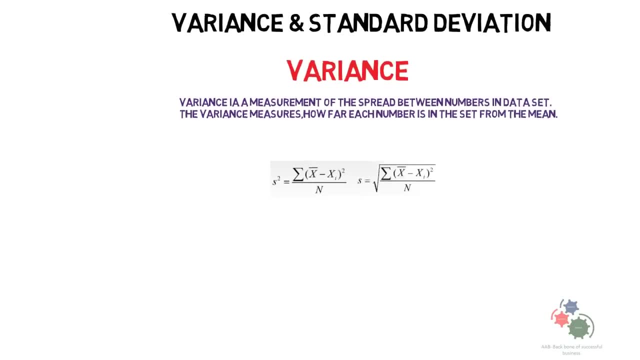 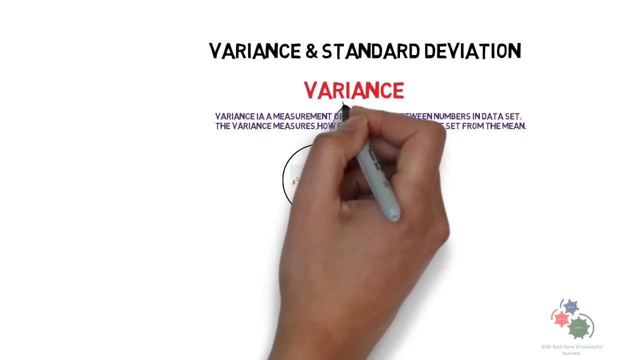 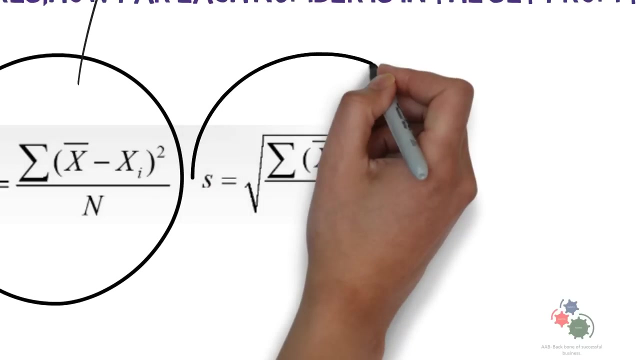 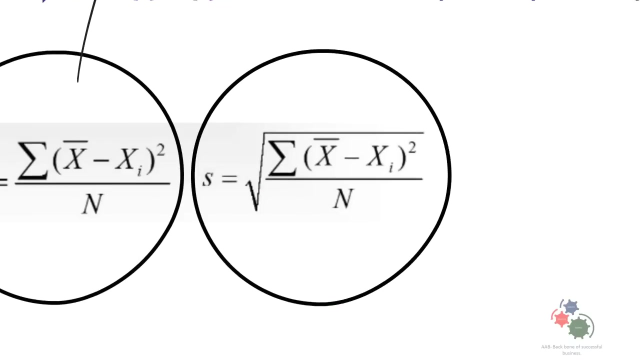 The variance measures how far each number in the dataset is from the mean. If you see equation below: here s square is variance equals to summation of x bar minus minus x square by n. Standard Deviation: S denotes standard deviation. Standard deviation equation is root over summation of x bar minus x whole square by n. 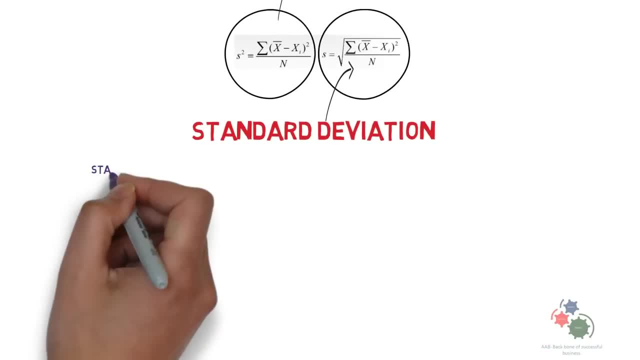 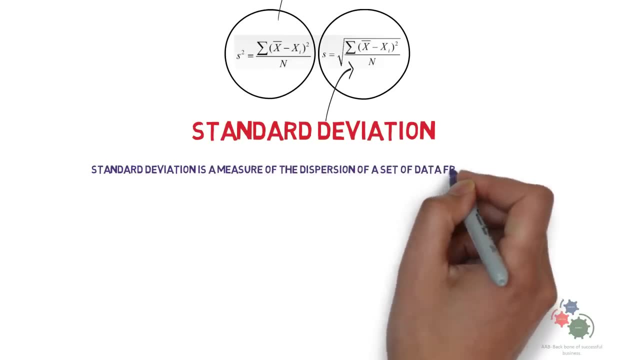 In other words, we can say standard deviation is root over of variance. We can say standard deviation is a measure of the distribution Dispersion of a set of data from the mean. It is calculated as the square root of variance by determining the variation between each. 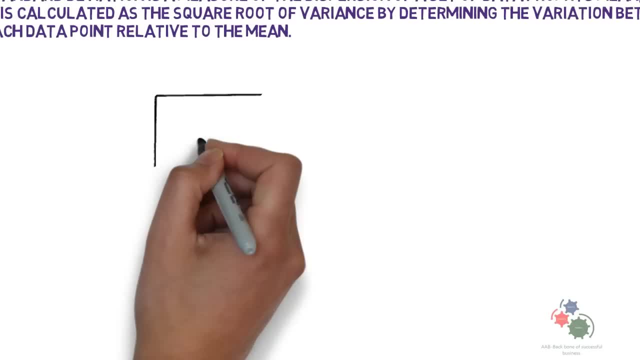 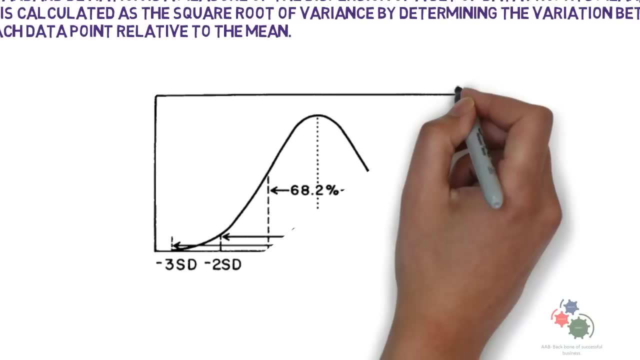 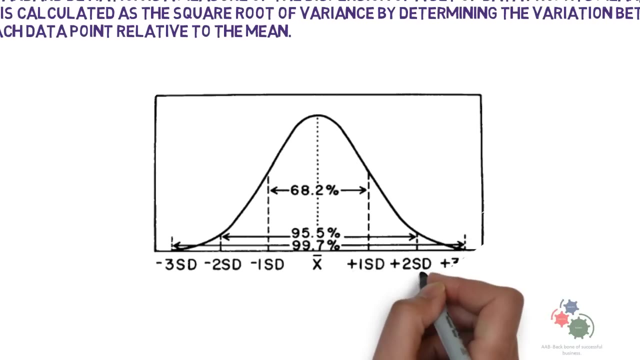 data point related to the mean. We can explain standard deviation by below-valve curve. Here: one standard deviation is 68.2 percent. Two standard deviation is 95.5 percent. Three standard deviation is 90.5 percent. Four standard deviation is 95.2 percent. 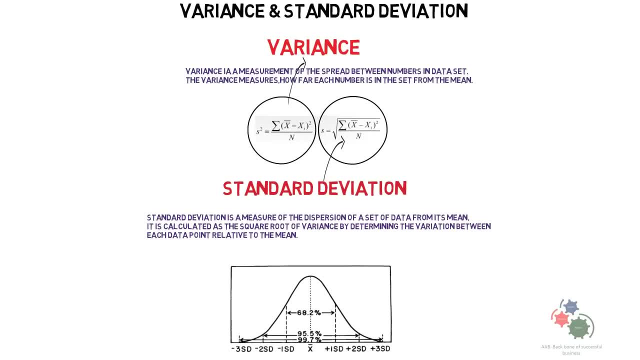 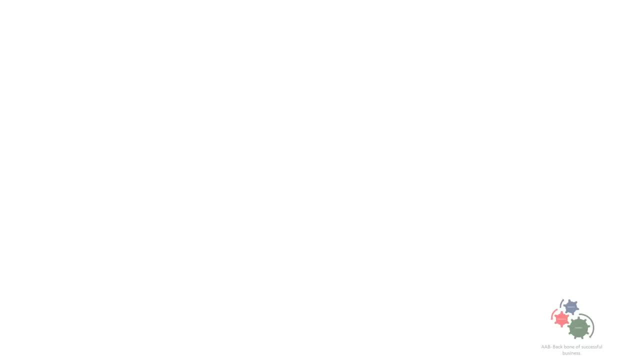 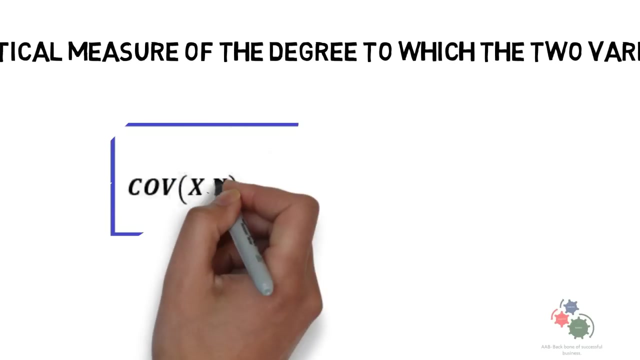 Three: standard deviation is 90.5 percent. C standard deviation is 99.7%. Covariance and Correlation Coefficient. Covariance: Covariance is a statistical measure of the degree to which the two variables move together. Let's understand by below formulae: 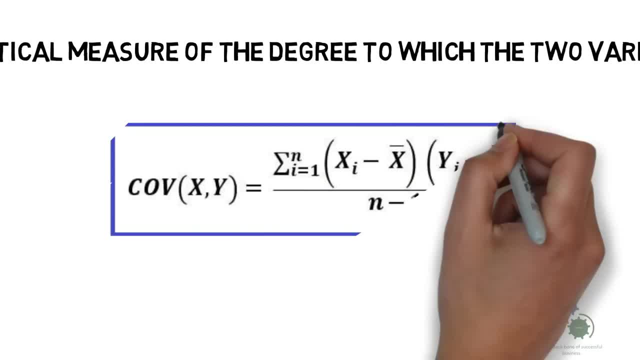 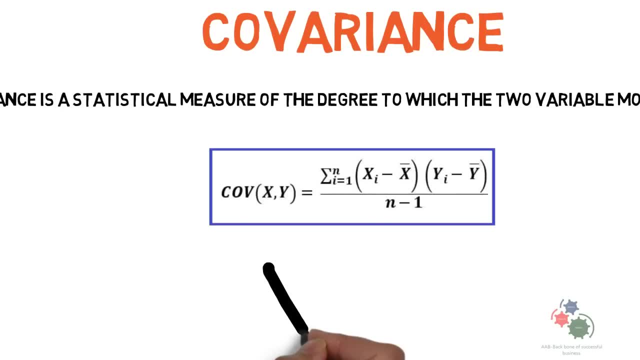 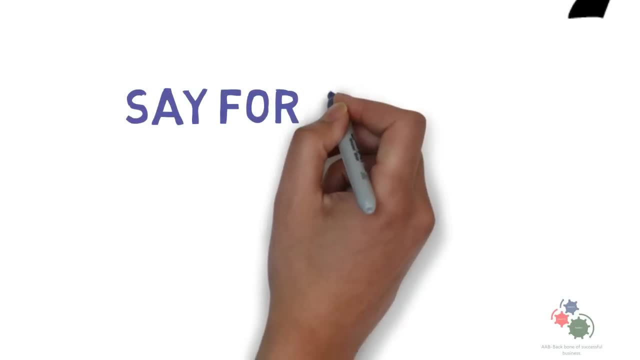 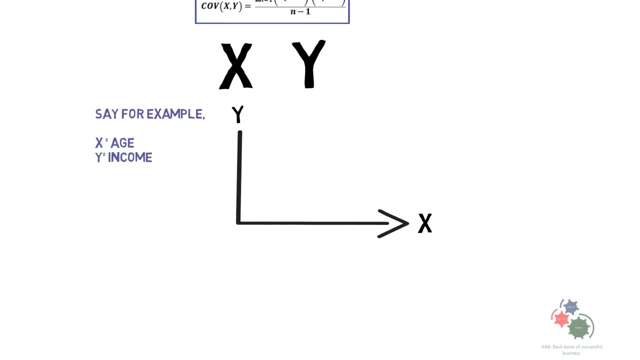 Covariance. xy is equal to x minus x bar into y minus y bar divided by n minus 1.. Here we are talking about two variables, x and y. Say for example: x is equal to age, y is equal to income. As age is increasing, y also increasing. 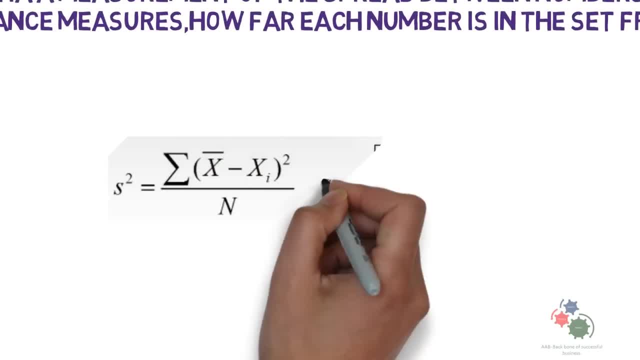 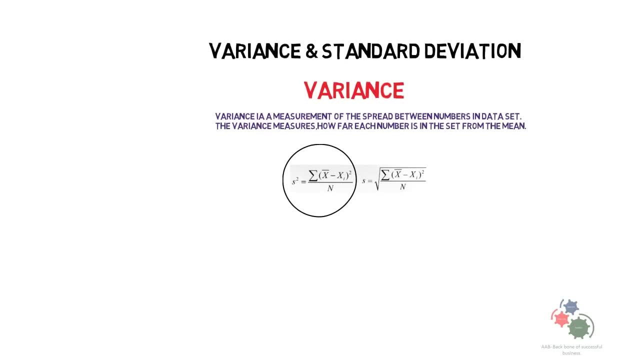 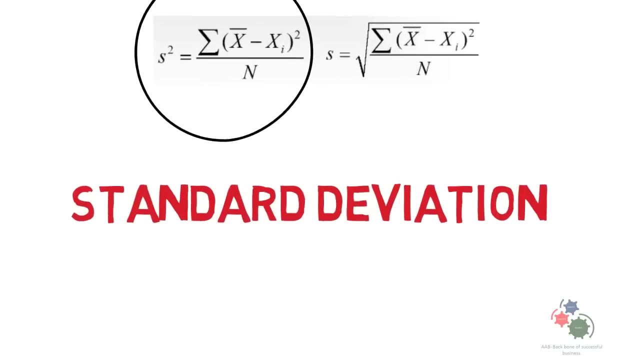 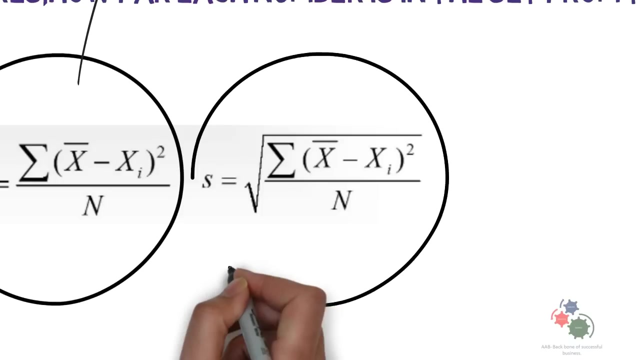 the sample. If you see equation below here: S square is variance equals to summation of x bar minus x, square by n. Standard deviation S denotes standard deviation. Standard deviation equation is Root over summation of x bar minus x whole square by n. 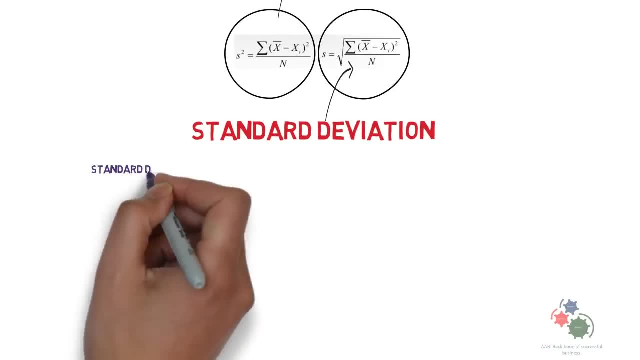 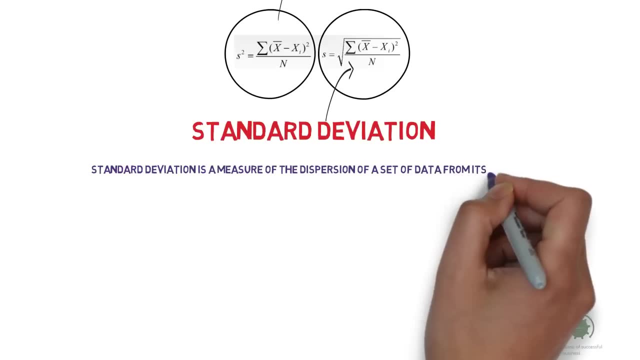 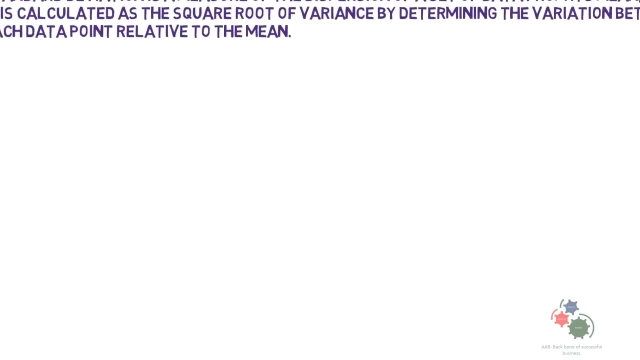 For example, we can say standard deviation is root over of variance. We can say standard deviation is a measure of the dispersion of a set of data from the mean. It is calculated as the square root of variance by determining the variation between each data point related to the mean. 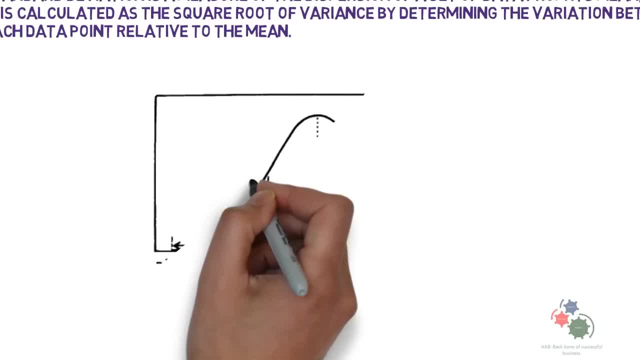 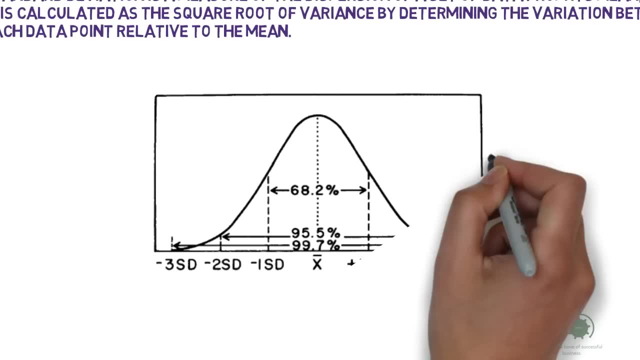 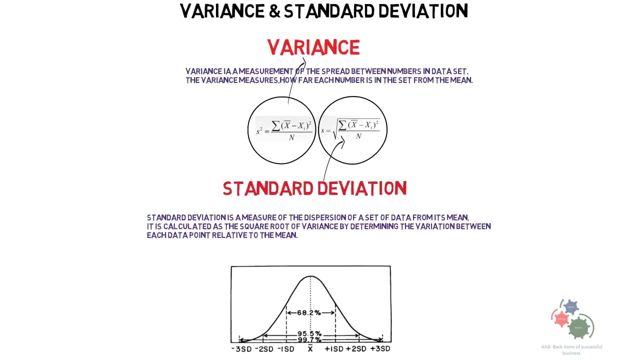 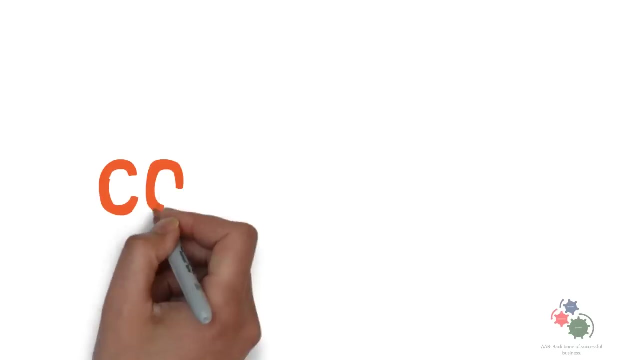 We can explain standard deviation by below. well, curve Here. one standard deviation is 68.2%. two standard deviation is 95.5%. three standard deviation is 99.7%. Covariance and Correlation Coefficient. Covariance. Covariance is a statistical measure of the 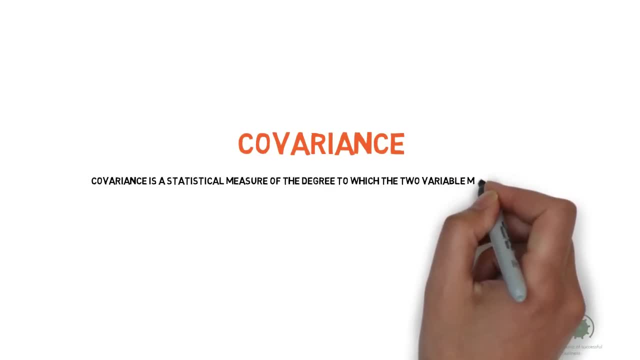 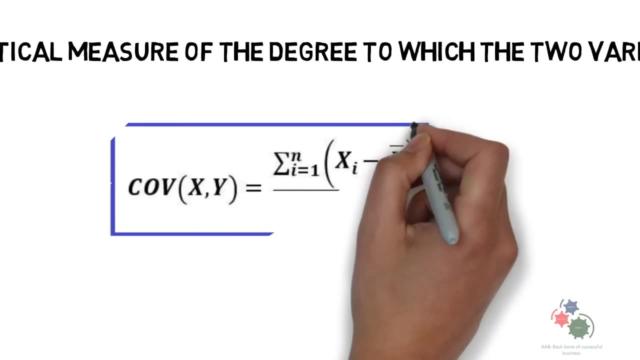 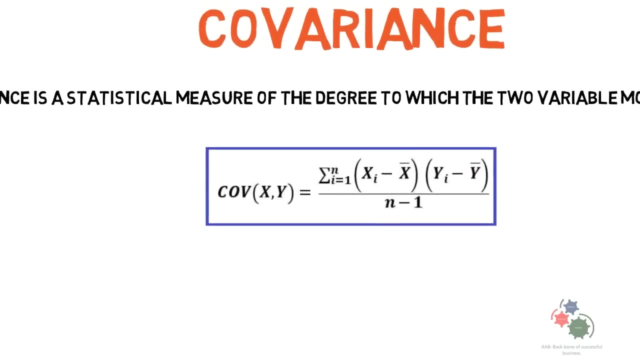 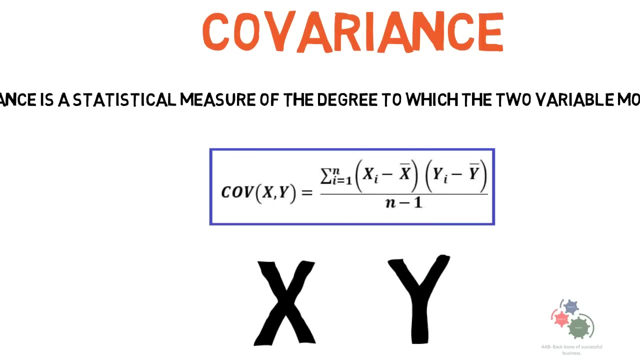 degree to which the two variables move together. Let's understand by below formulae: Covariance is what Covariance is equal to. We are talking about two variable, X and Y. Say, for example, X is equal to Age, Y is equal to Income. 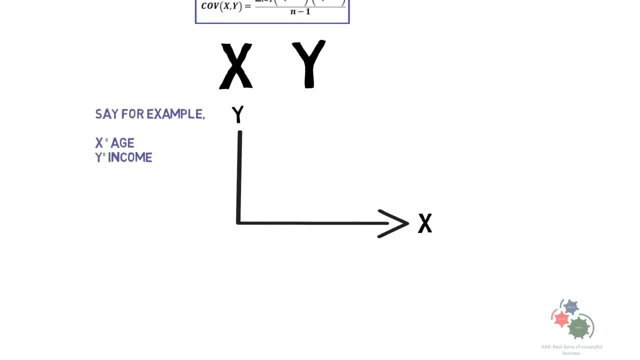 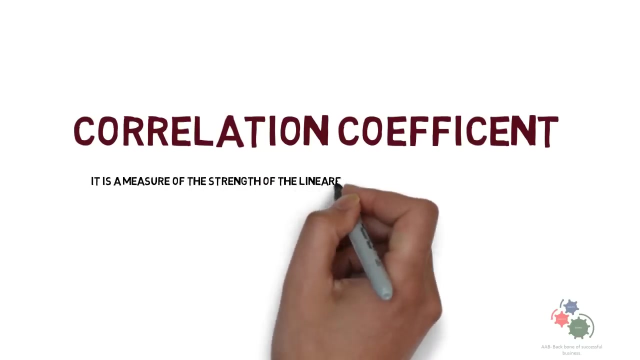 airs. H, y is equal to Income. 聽л hear, tighten the books. If you wish, you can check the description box below. As h is increasing, y also increasing. That is called positive relationship Correlation coefficient. It is a measure of the strength of the linear relationship between two variables. 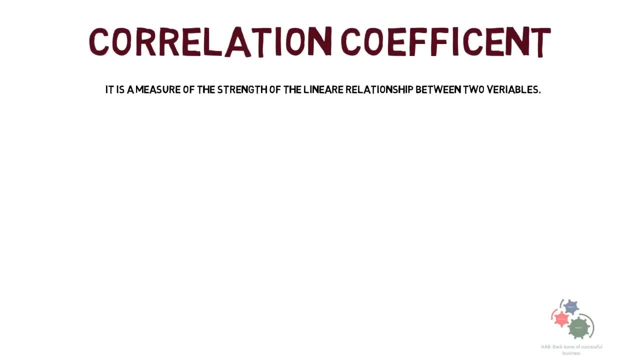 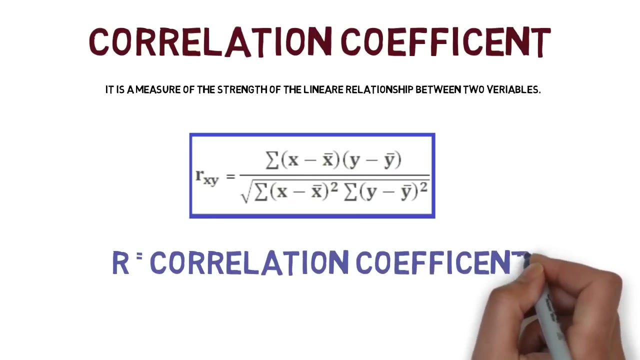 Let's understand it by below formulae: Summation of x minus x bar into y minus y bar, divided by root over summation of x minus x bar whole square into summation of y minus y bar whole square. Correlation coefficient denoted by r. 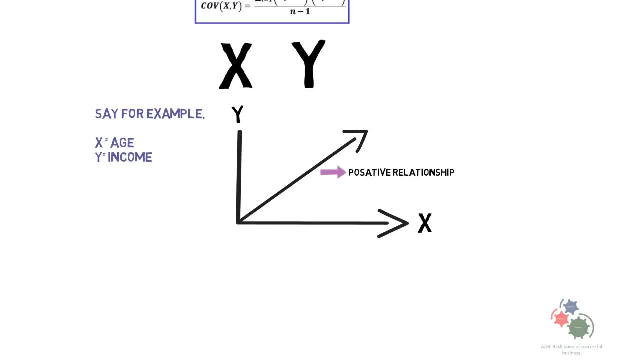 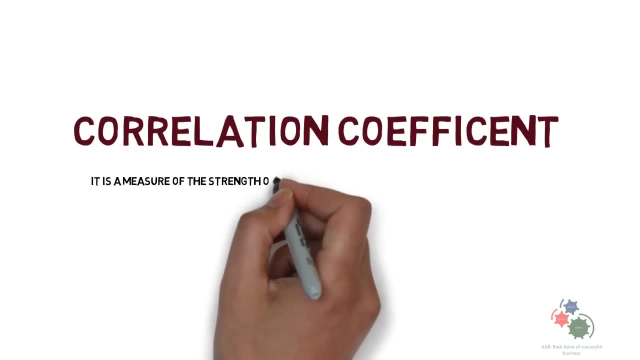 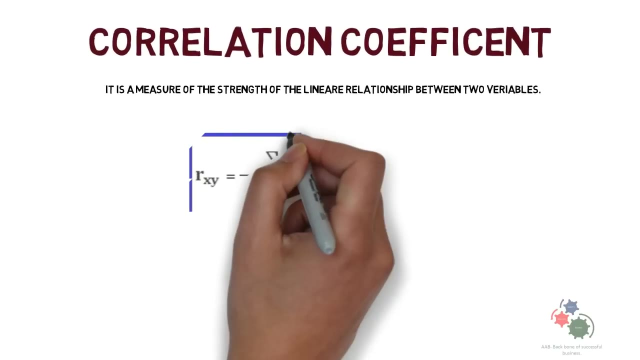 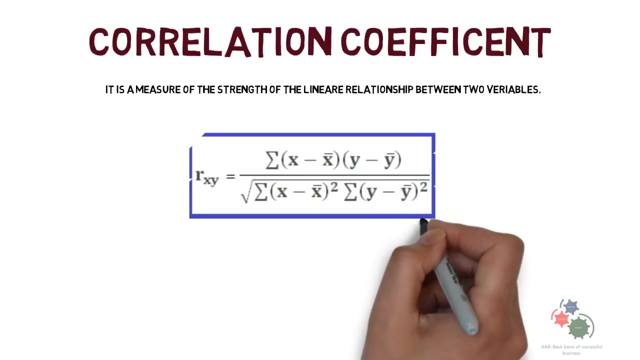 That is called positive relationship Covariance Correlation coefficient. It is a measure of the strength of the linear relationship between two variables. Let's understand it by below formulae: Summation of x minus x bar into y minus y bar divided by root over summation of x minus. 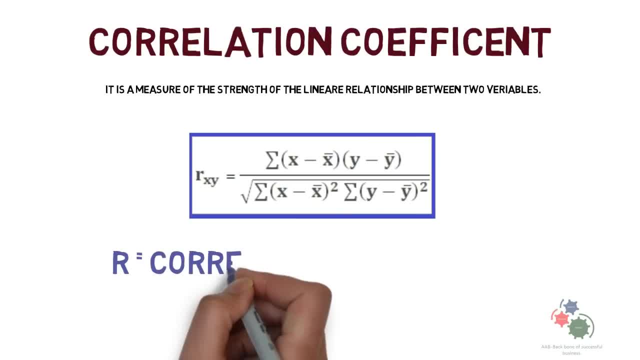 x bar whole square into summation of y minus y bar whole square. Summation of x minus x bar into y minus y bar whole square. Summation of x minus x bar into x bar whole square. Summation of x minus x bar into x bar whole square. 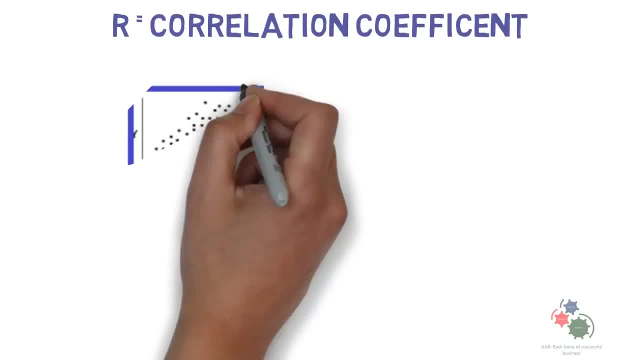 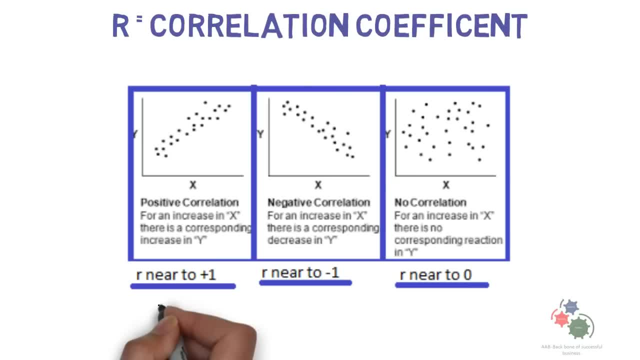 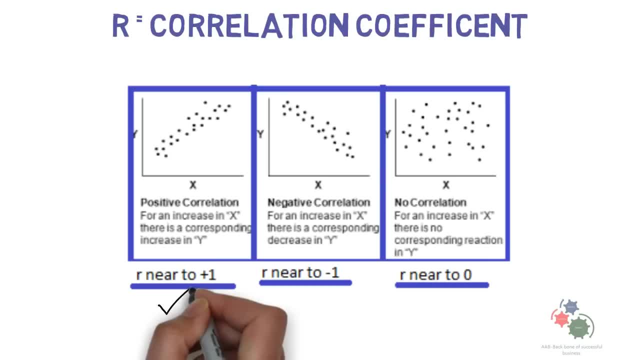 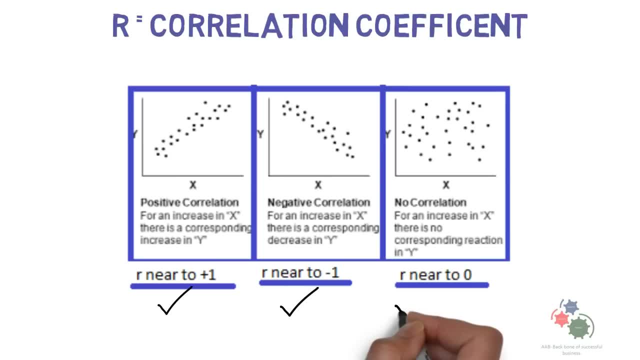 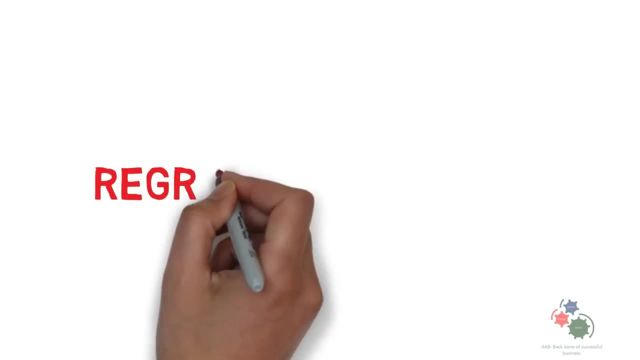 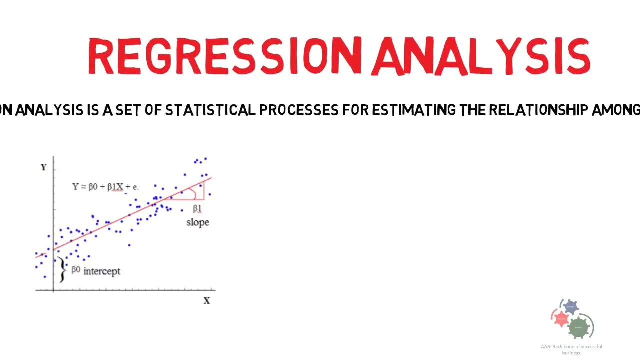 negative correlation. in this plot. for an increasing of x there is no correspondent reaction in y. here no correlationship is existing regression analysis. regression analysis is a set of statistical process for estimating the relationship among variables. let's understand it by below graph and equation. here beta 0 is intercept. 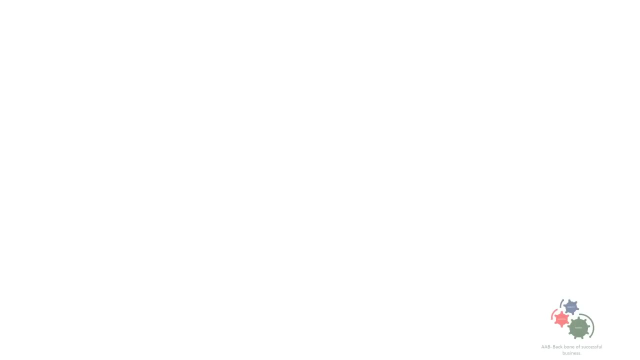 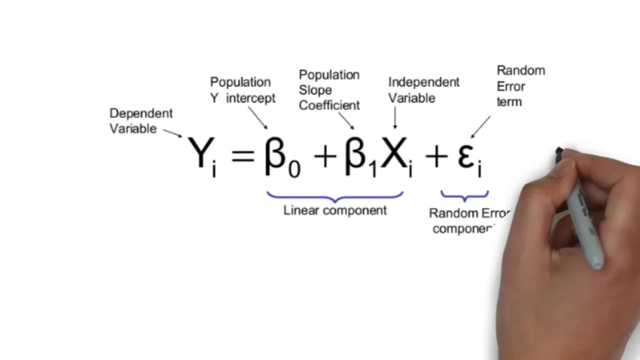 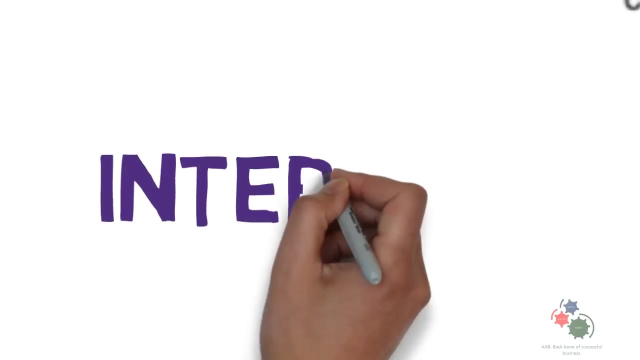 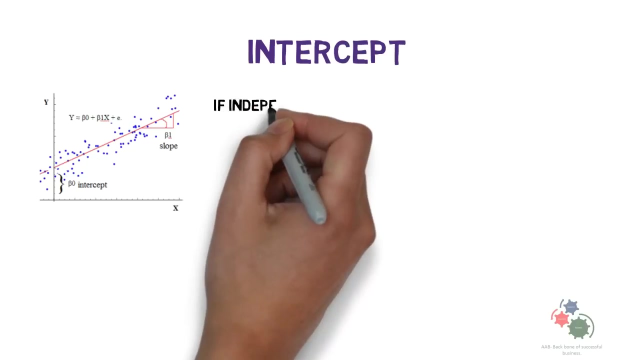 beta 1 is slope coefficient. in this equation, y is dependent variable. beta 0 is intercept. beta 1 is slope coefficient. x is independent variable. e is random error. let's understand intercept if independent variable does not move. now how muchnosis happened? independent variable. let's checking the data. 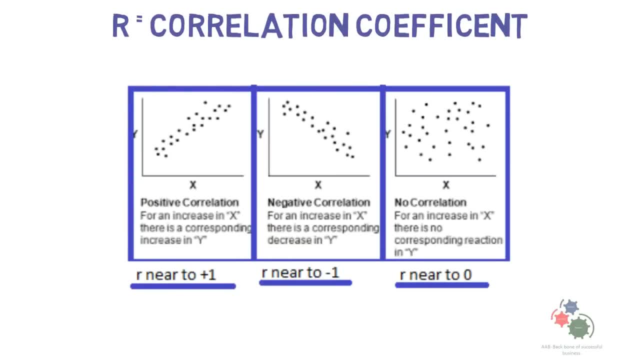 Let's understand correlation coefficient by below plots. Here: as h is increasing, As h is increasing, y also increasing. That is called positive correlation. Here, as h is increasing, y is decreasing. It is the example of negative correlation. In this plot for an increasing of x, there is no correspondent reaction in y. 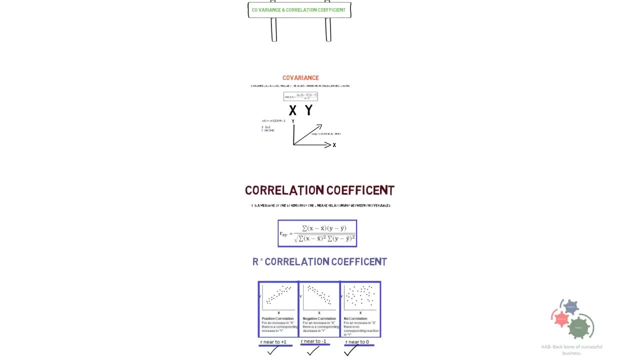 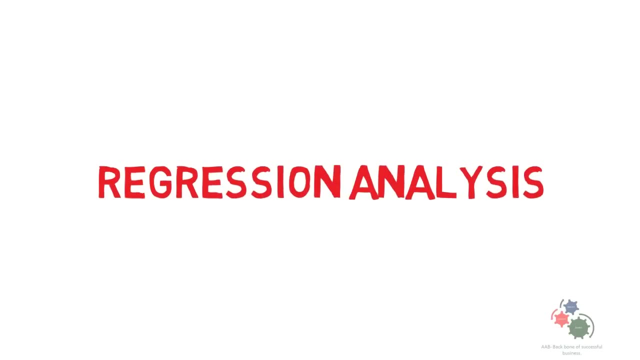 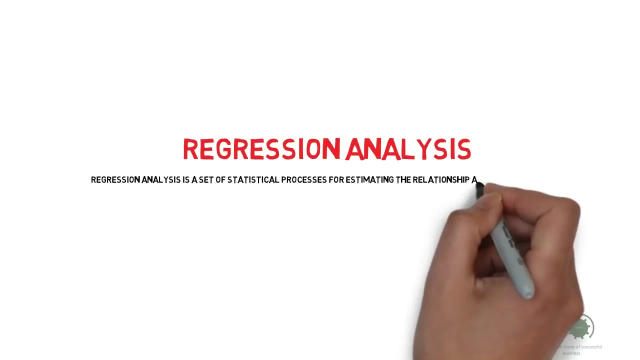 Here no correlation is existing. It is the example of negative correlation. Regression analysis. Regression analysis is a set of statistical process for estimating the relationship among variables. Regression analysis is a set of statistical process for estimating the relationship among variables. Let's understand it by below graph and equation. 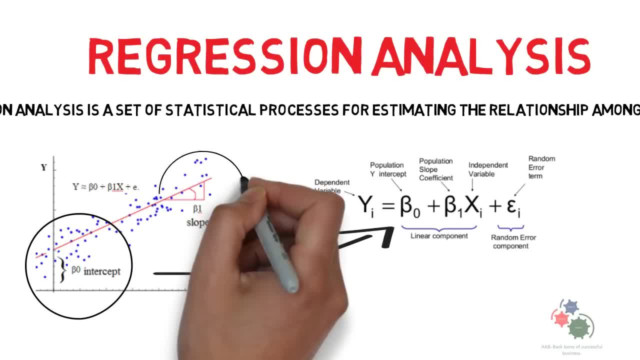 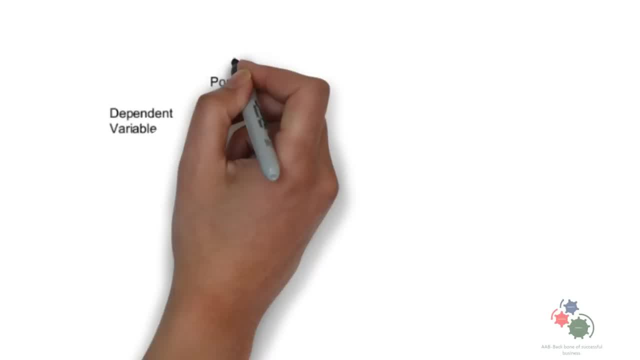 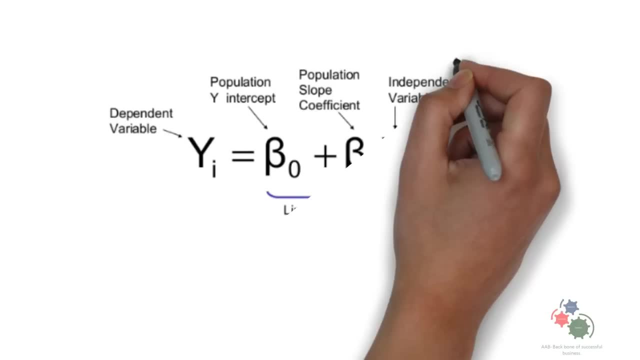 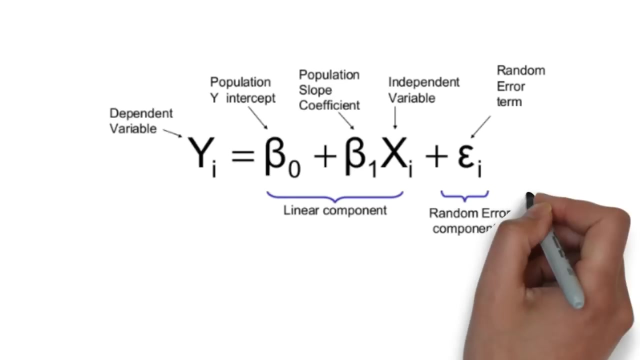 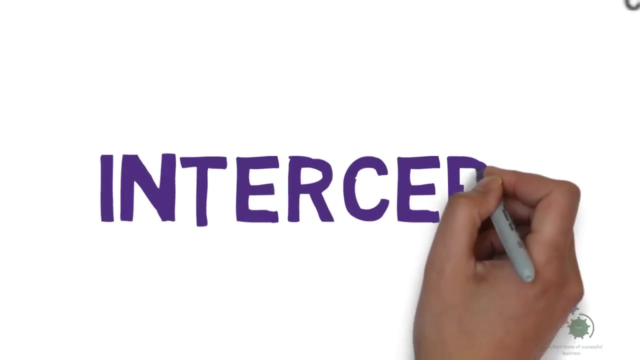 Here, beta 0 is intercept, Beta 1 is slope coefficient. In this equation, Y is dependent variable, beta 0 is intercept. beta 1 is slope coefficient. X is independent variable. E is random error. Let's understand intercept. 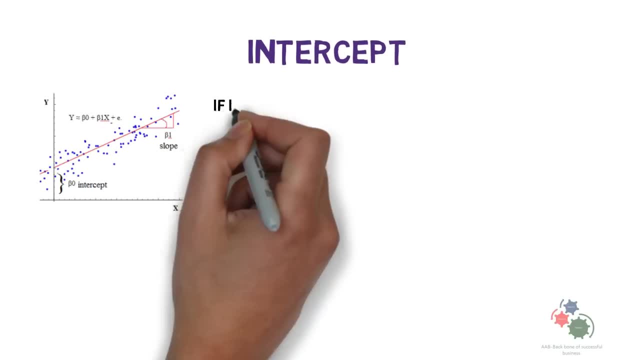 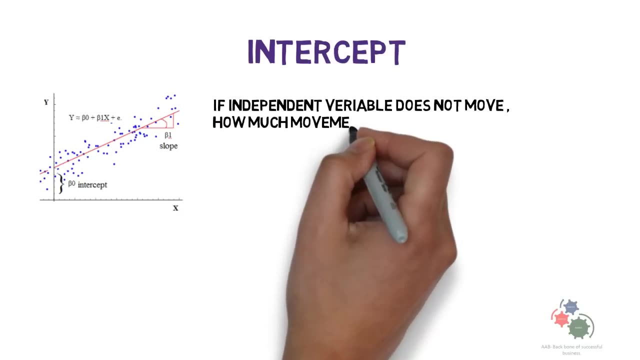 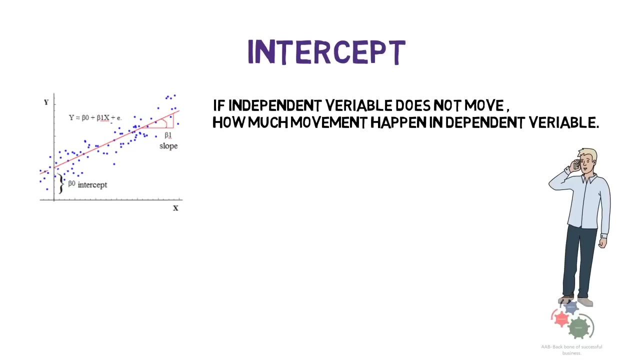 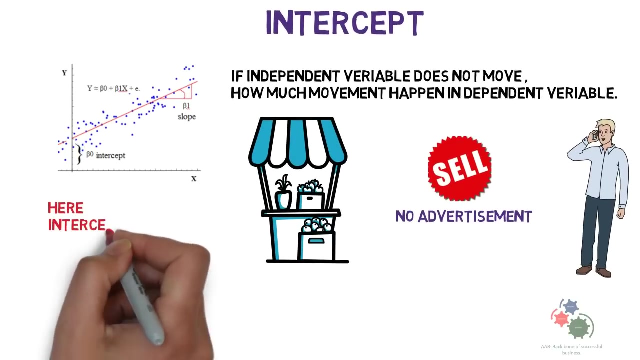 If independent variable does not move, how much change happen in dependent variable? Let's understand it by below example. You open a new shop. You realize some best sales is happening without doing any advertisement. Here intercept is baseline sales, X is equal to advertisement, Y is equal to sales. 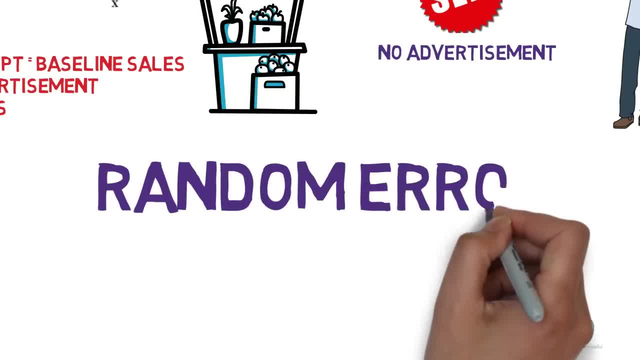 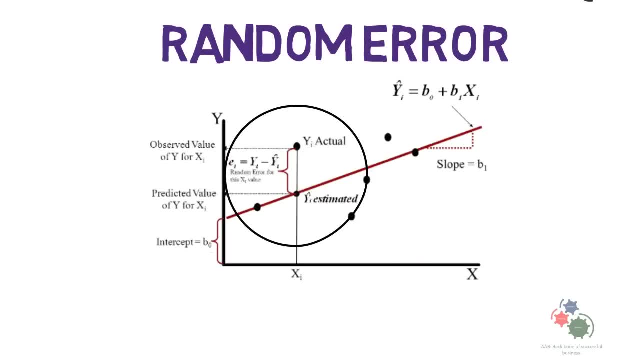 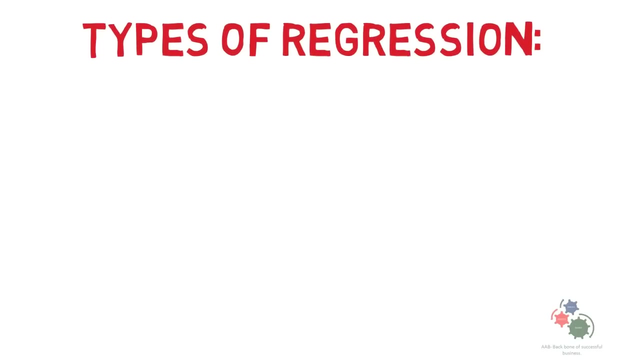 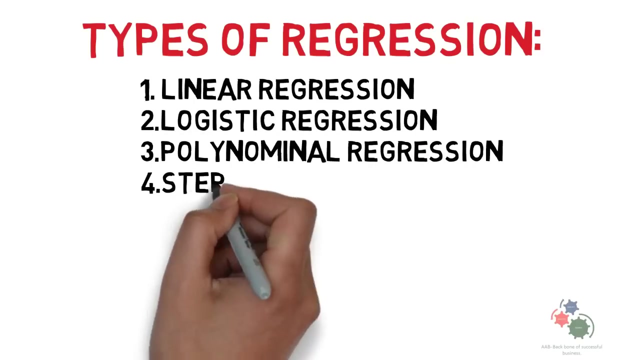 Now let's understand random error Here. YI is actual value of Y, Y hat is estimated value of Y. So random error is actual, minus estimated. Types of regression: Linear regression, logistic regression, polynomial regression, stepwise regression, rigid regression. 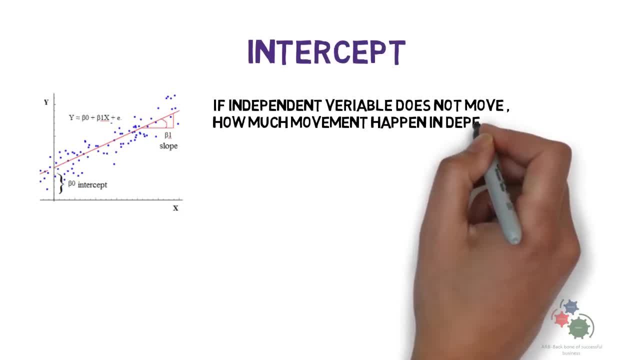 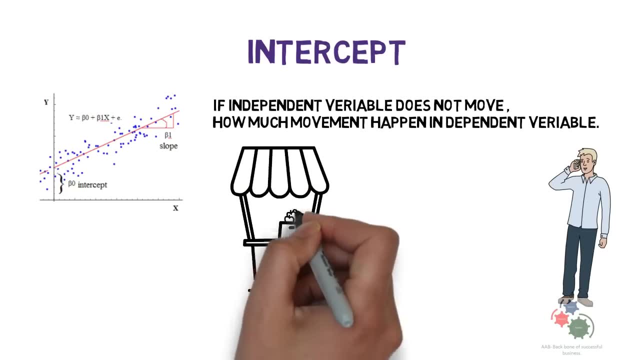 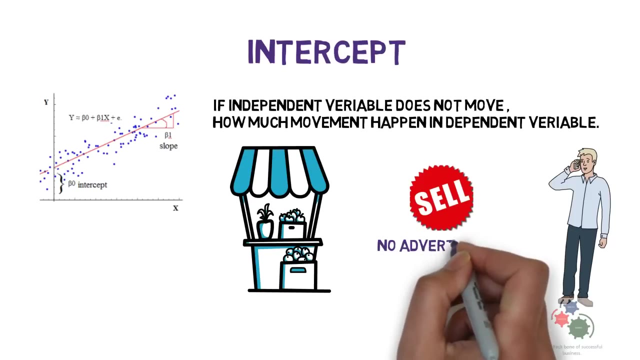 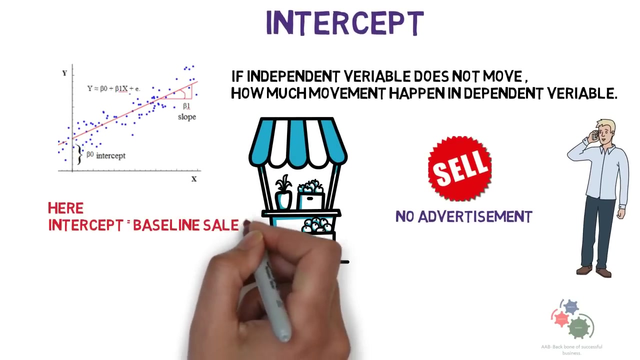 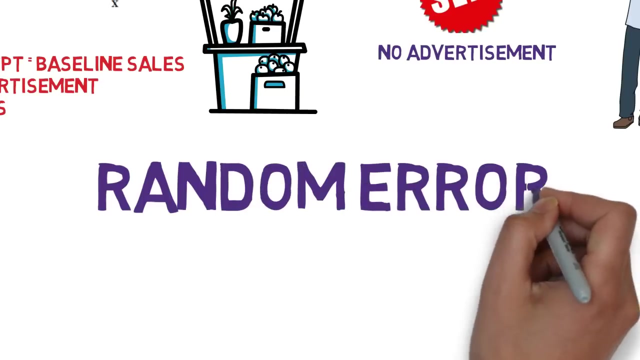 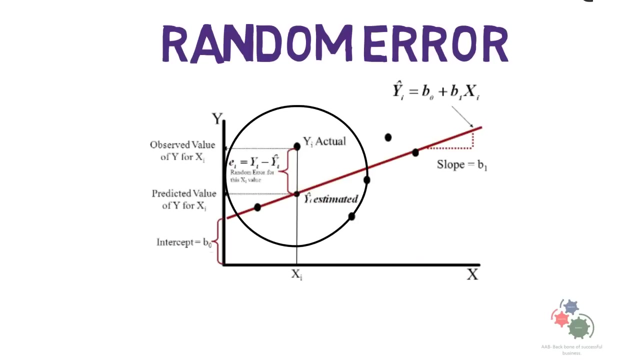 details in an example. you open a new shop, you realise beta will increase. base sales is happening without doing any advertisement. here intercept is baseline sales. X is equal to advertisement, Y is equal to sales. Now let's understand random error Here. YI is actual value of Y, Y hat is estimated value of Y. 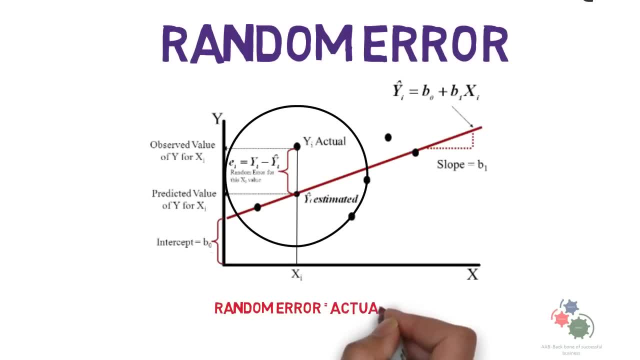 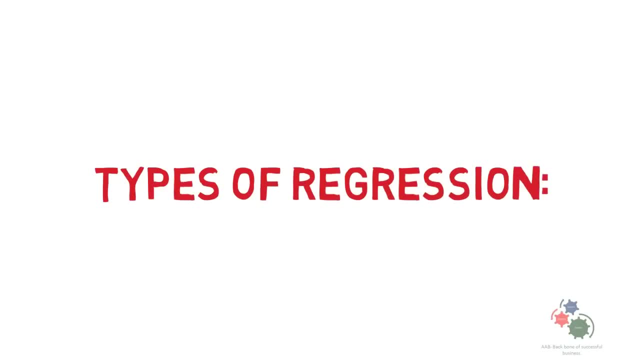 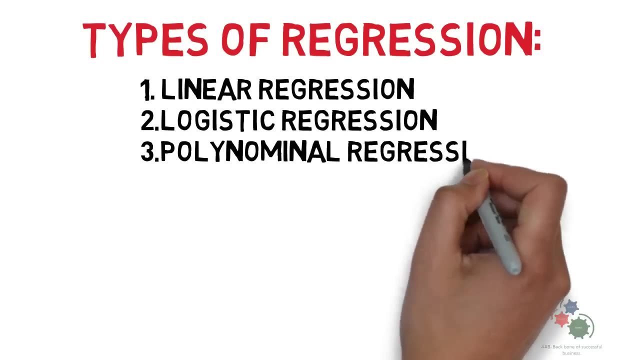 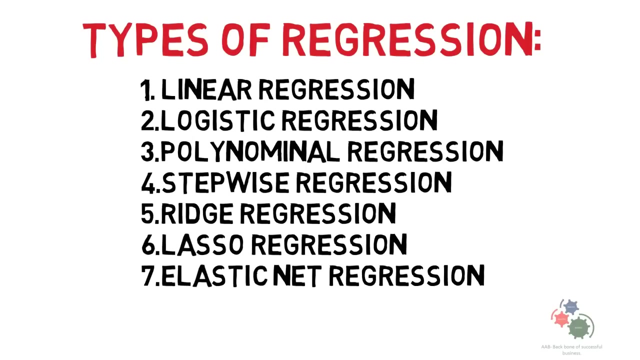 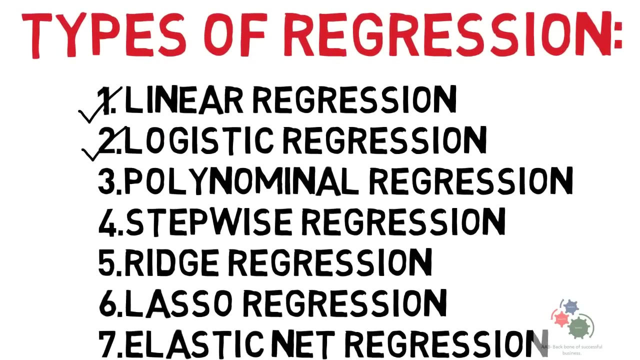 So random error is actual minus estimated. Types of regression: Linear regression, Logistic regression, Polynominal regression, Stepwise regression, Rigid regression, Lasso regression, Elastic net regression, Linear regression, Logistic regression are most used technique in business analytics. 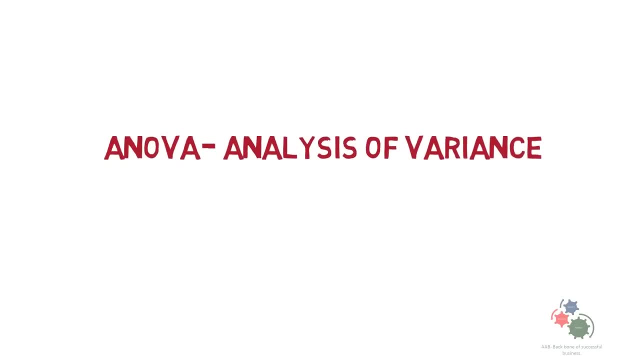 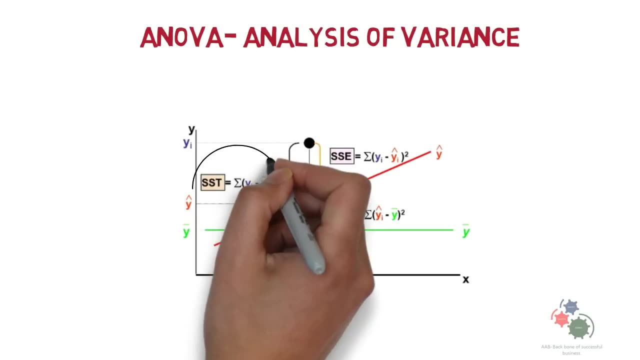 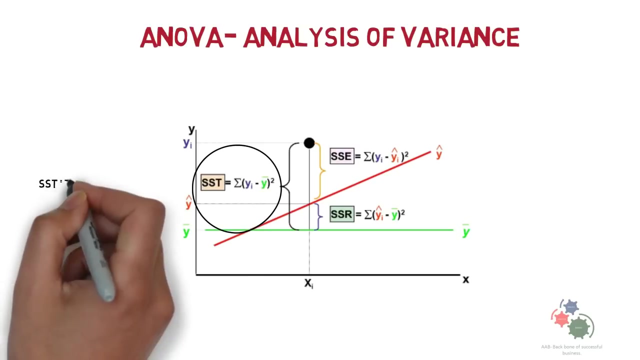 ANOVA. Analysis of Variance. Let's understand the concept, Let's brighter. based on number of mitigations. Let's answer these funnel questions Here. summation of actual value of Y minus format of Y: whole squared equals to total sum of squares. sum of equal parts equals to total sum of squares. 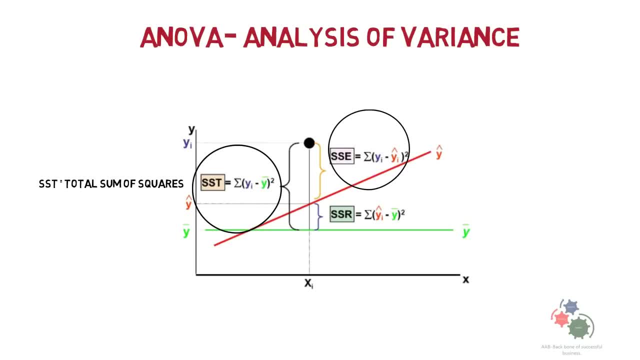 Next, if we focus on this part, Sum of square. Now, this part, summation of predicted y minus mean of y, whole square, equals to SSR Regression Sum of Square, also known as Sum of Square Regression SSR. So we can say SST. 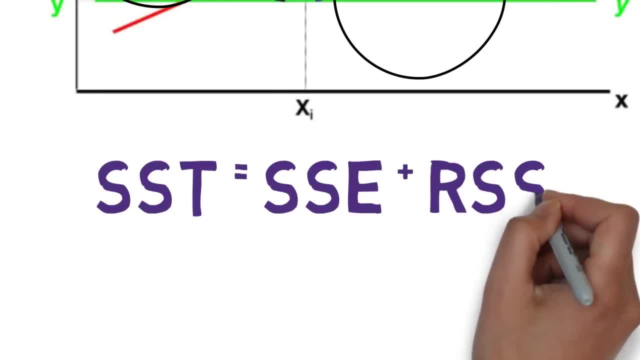 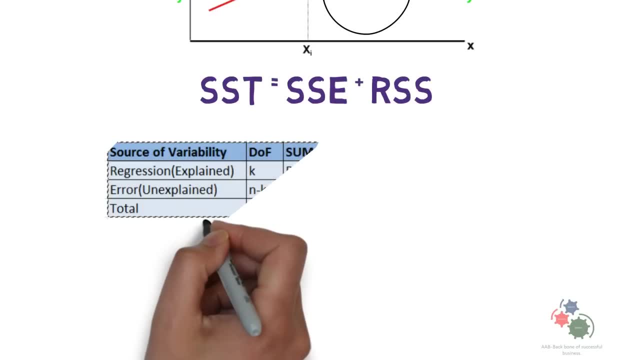 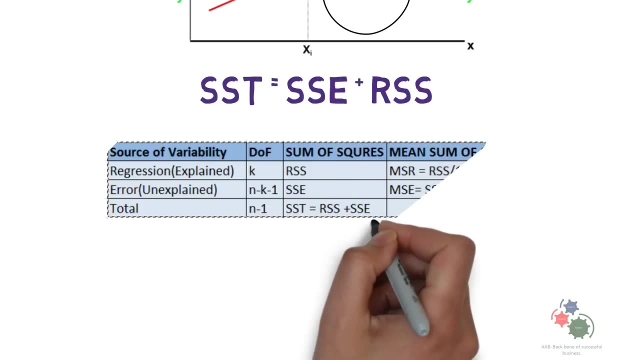 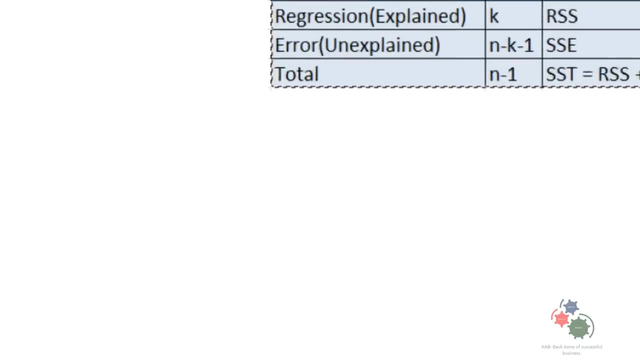 equal to SSE plus RSS. Sum of Square is SSE. Mean Sum of Square MSE is equal to SSE by N by 2.. Total Degrees of Freedom: N minus 1, Sum of Square STT equal to RSS plus SSE. Standard Error of Estimate Root over MSE. Root over SSE by N minus 2.. 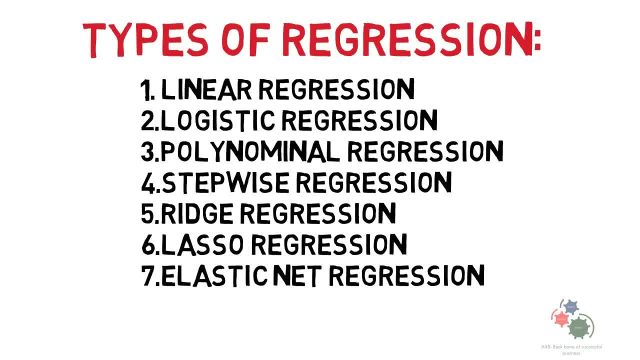 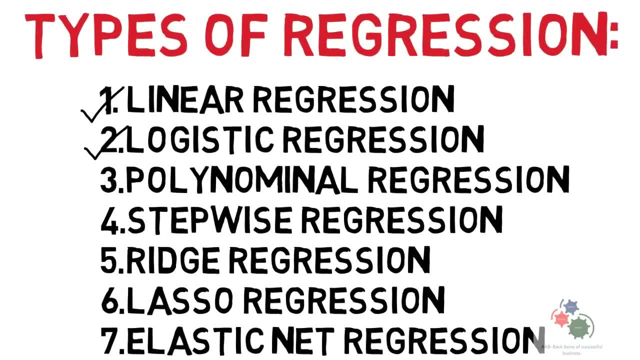 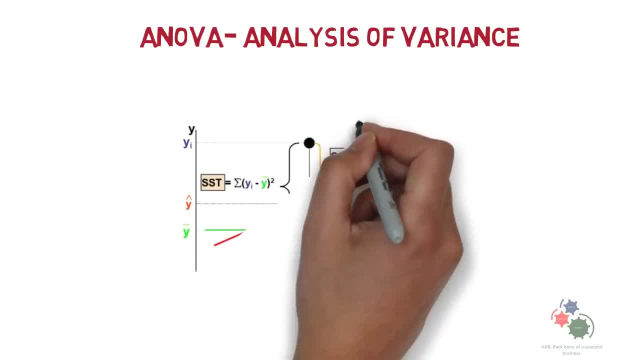 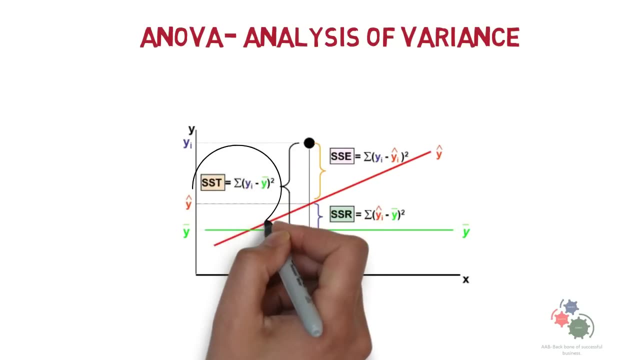 lasso regression, elastic net regression, linear regression, logistic regression are most used technique in business analytics: ANOVA analysis of variance. Let's understand the concept of variance. Let's understand the concept of variance Here, the term 토�. 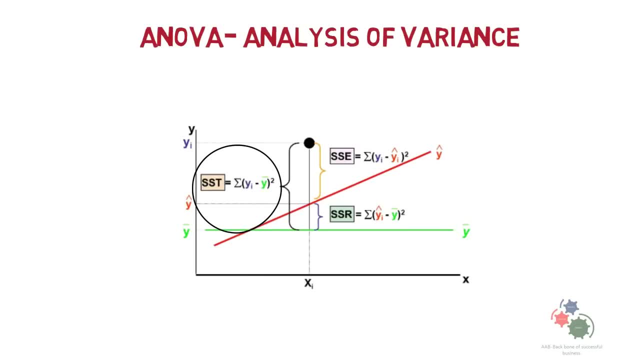 Summation of actual y minus mean of y whole square: IЛM, SST. Summation of actual y minus predicted y whole square is SSE. serum error Sum on the day before fixation: IML, SI, I incrop, PS, Z, IEO, SS, П. 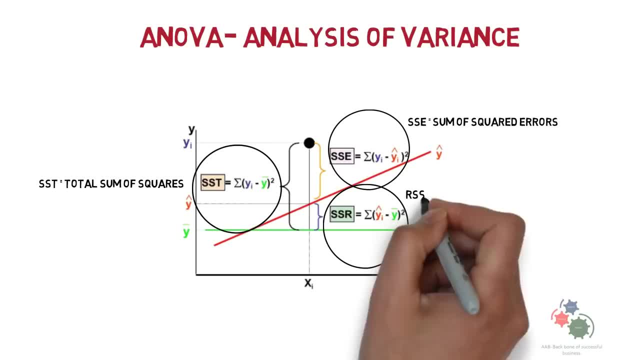 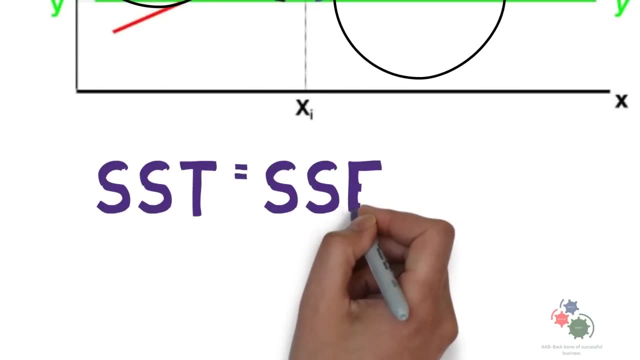 Augment of totalsti terms. What's normale summary EfR Summation of predicted y minus mean of y: whole square equals to SSR regression sum of square, also known as sum of square regression SSR. So we can say SST equal to SSE plus RSS. 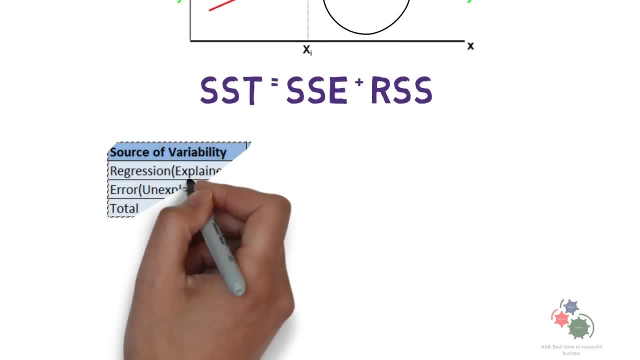 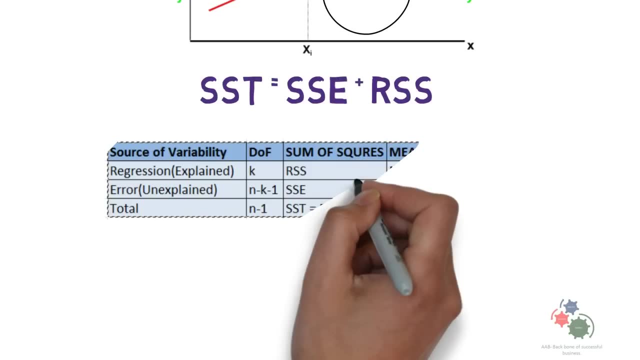 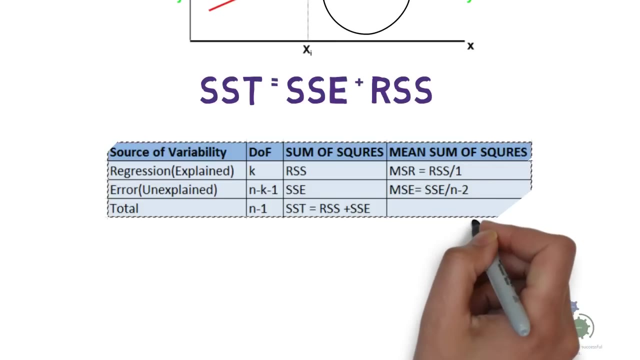 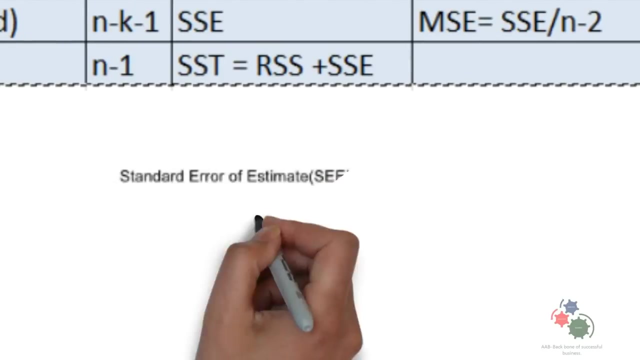 Sum of square is SSE. mean sum of square MSE is equal to SSE by n by 2.. Total degrees of freedom: n minus 1,. sum of square SST equal to RSS plus SSE. standard error of estimate: root over MSE. root over SSE by n minus 2.. 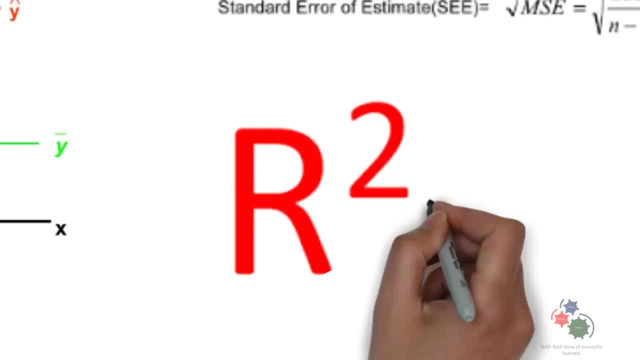 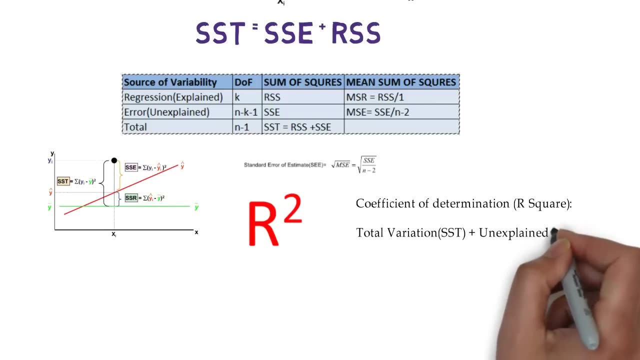 Now most important topic: R square Coefficient of determination. R square, Total variation SST plus unexplained variation SSE Divided by total variation. Total variation SST. Exchanged variation RSS divided by total variation SST. 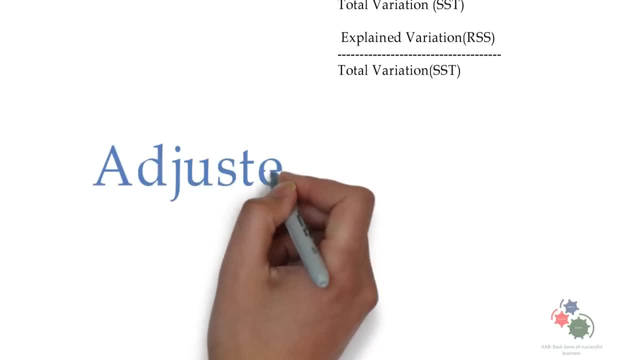 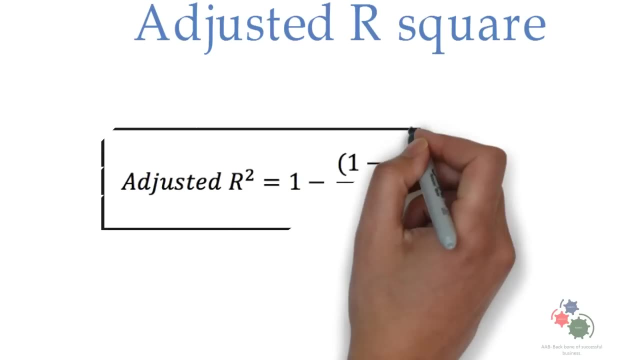 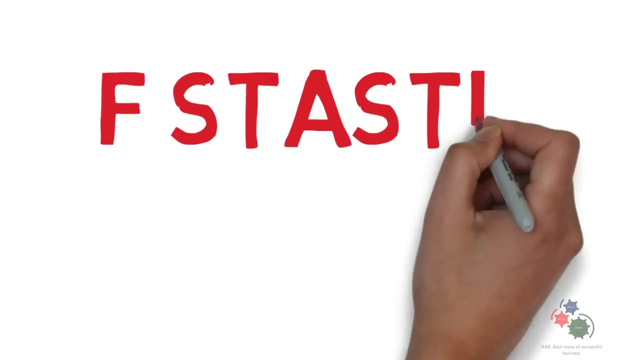 Next topic is adjusted R square. Adjusted R square equal to 1 minus 1 minus R square into n minus 1 divided by n minus p minus 1.. Now very important topic is F-statistics. An F-test explains how well the dependent variable is explained by the independent variable. 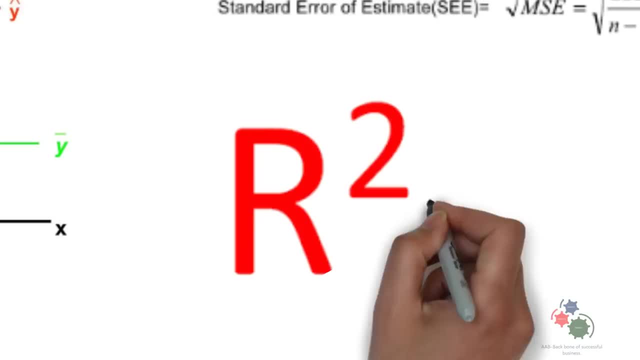 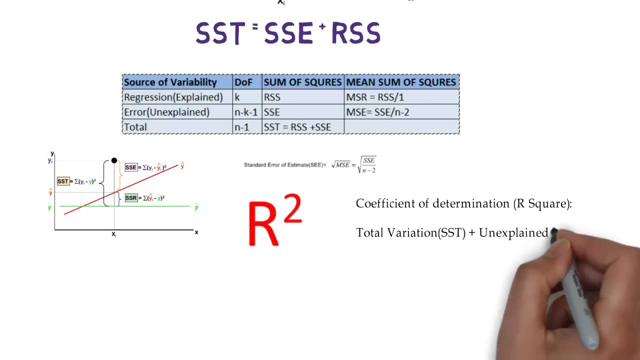 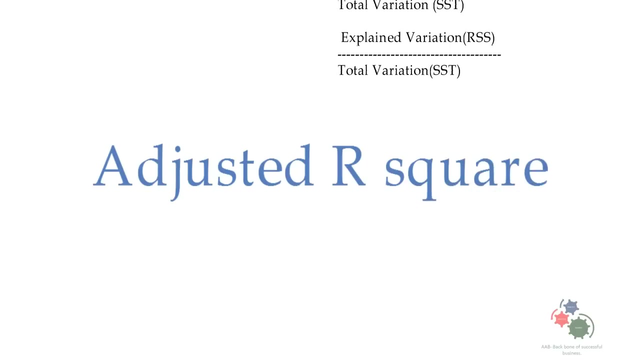 Now most important topic: R square. Coefficient of Determination R square. Total Variation STT. plus Unexplained лин variation SSE divided by Total Variation SST. Kardashian variation RSS divided by Total Variation SST. Next topic is Adjusted R square. Adjusted R square equal to 1 minus 1 minus. 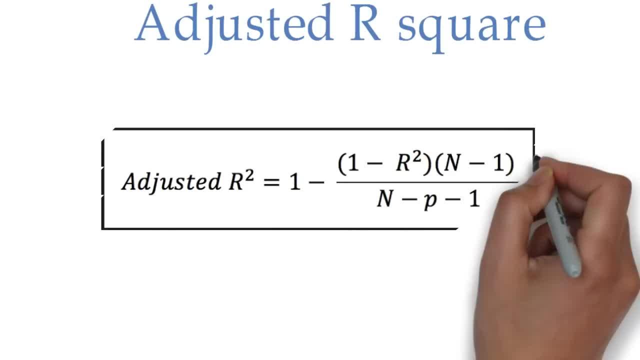 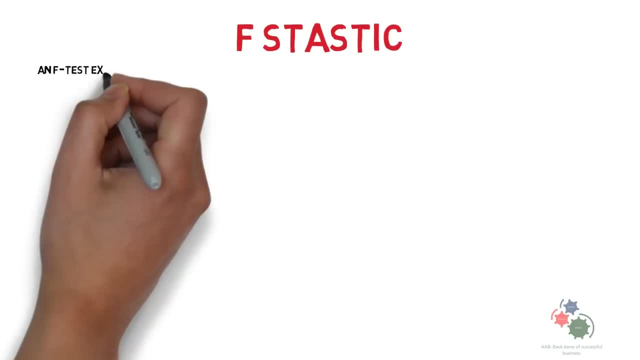 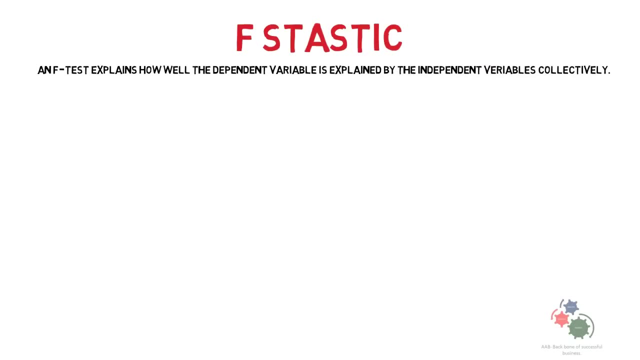 R square into N minus 1 divided by N minus p minus 1.. Now very important topic is F Statistic. An F test explains how well the Dependent variable is explained by the independent variables collectively. Here, MSR mean regression sum of squares, MSE mean square error, N. number of observation: K. 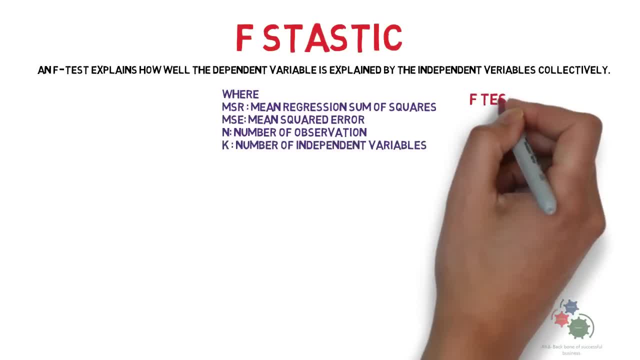 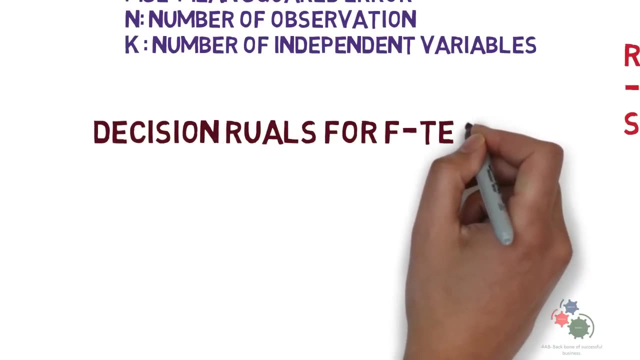 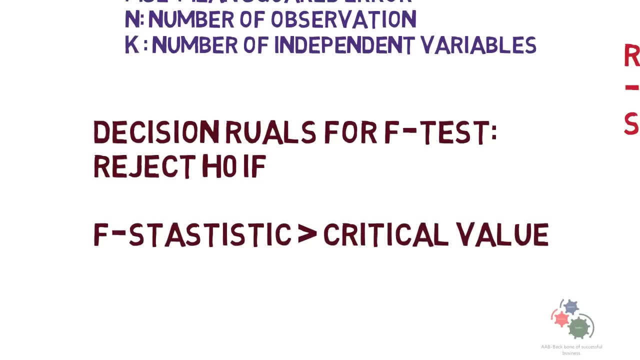 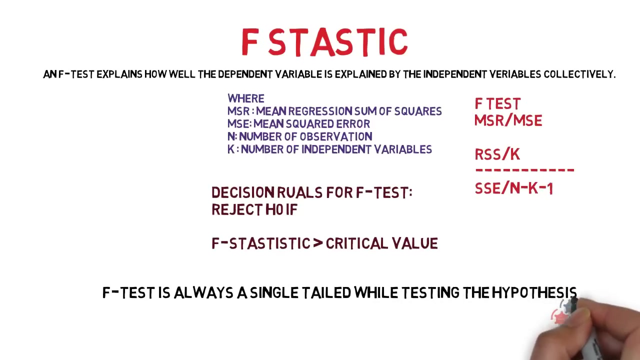 number of independent variables: F test: MSR divided by MSE, equal to RSS by K divided by SSE. divided by N minus K minus 1. decision rules for f test: Reject null hypothesis if F test is more than critical value. F statistics is always a single tailed while testing the hypothesis that the 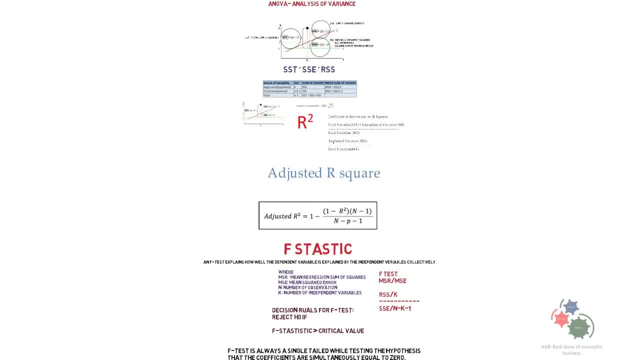 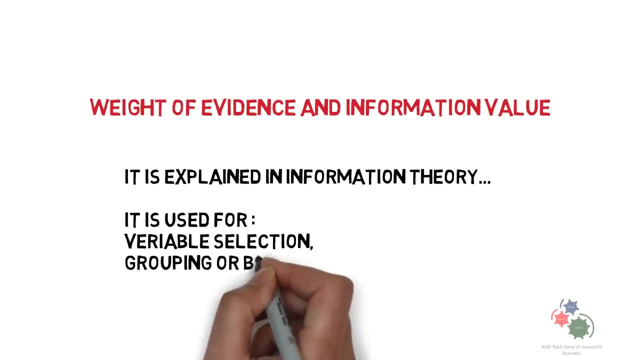 coefficients are simultaneously equal to zero. Our next topic is weightage of evidence and information value. It is explained in information theory. It is used for variable selection, grouping or binning variable predictive strength: more is weight, good is the variable. 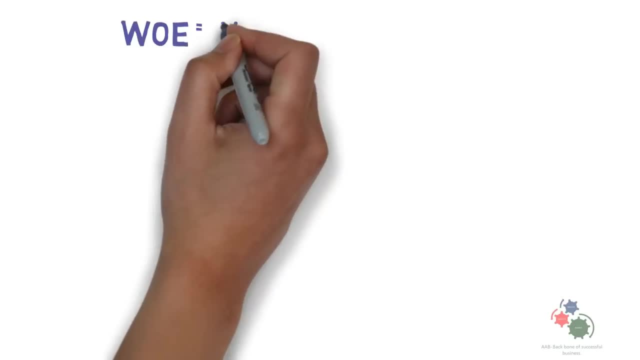 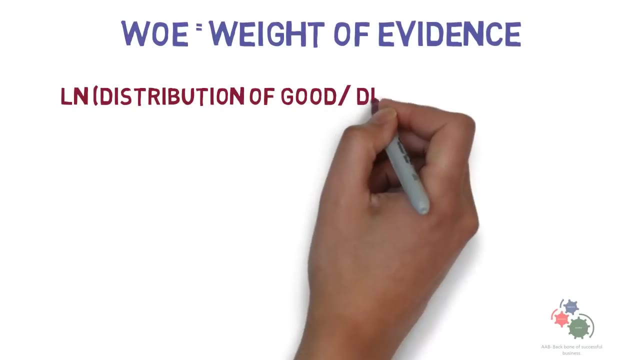 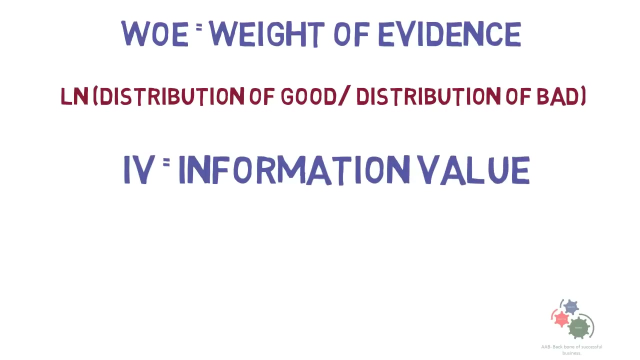 We can explain W O E, weightage of evidence, log of distribution of good by distribution of bad, IV information value, sum of distribution of good minus distribution of bad, into W O E, These two information mostly used in logistic regression. Let's understand the W O E. 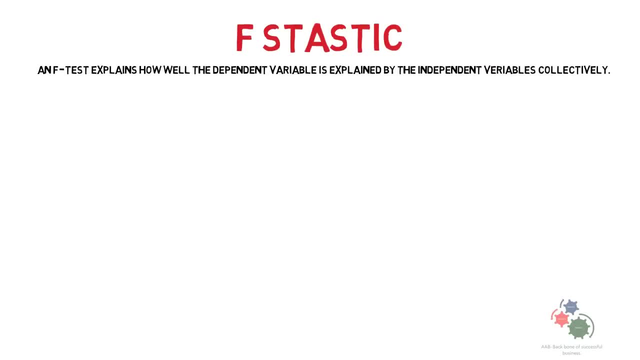 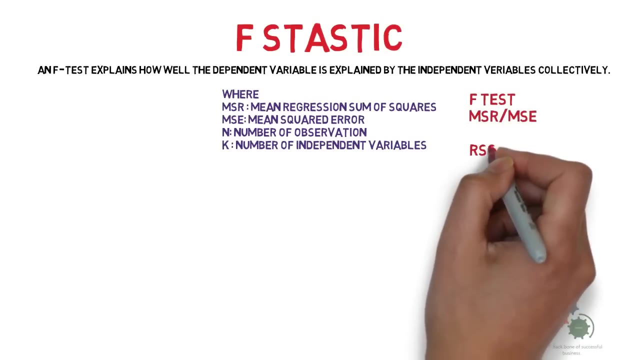 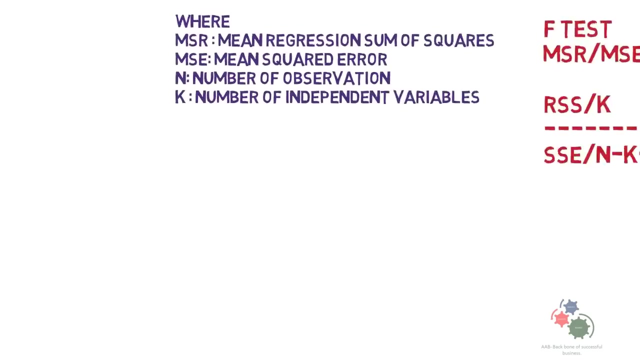 We use independent variables collectively. Here MSR mean regression sum of squares, MSE mean square error. N. number of observation. k. number of independent variables. F-test: MSR divided by MSE equal to RSS by k. divided by SSE, divided by n minus k minus 1.. 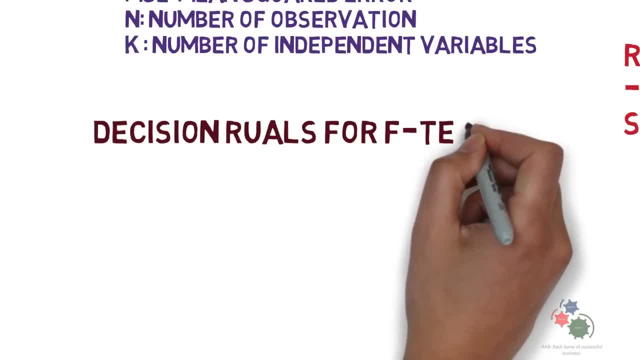 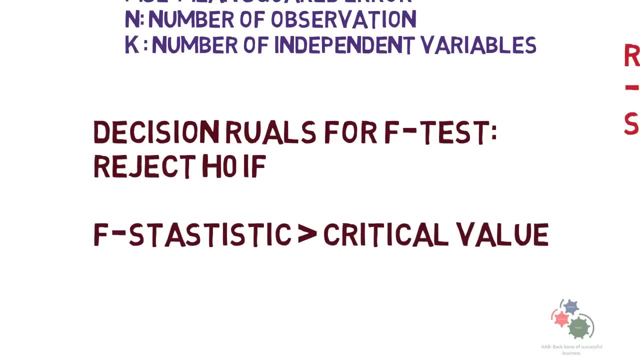 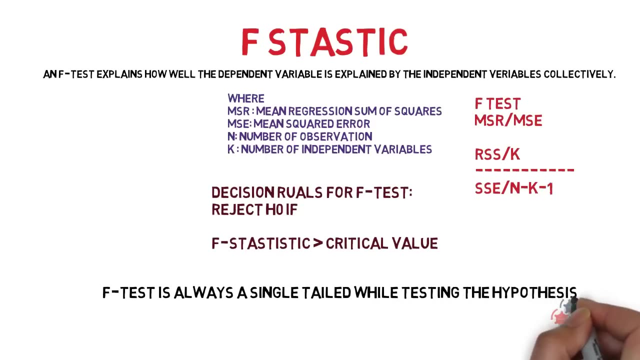 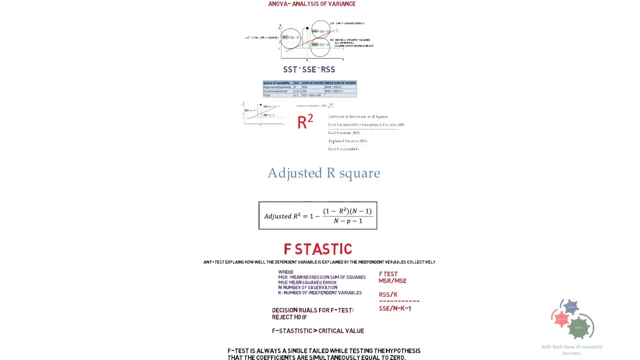 Decision rules for F-test. Reject Null Hypothesis if F-test is more than critical value. F-statistics is always a single-tailed while testing the hypothesis that the coefficients are simultaneously equal to zero. Our next topic is Quotient of Evidence and Information Value. 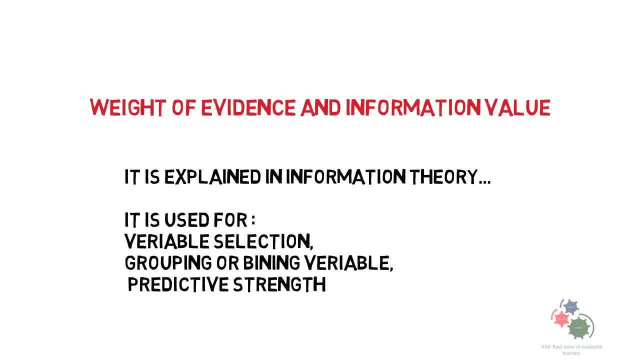 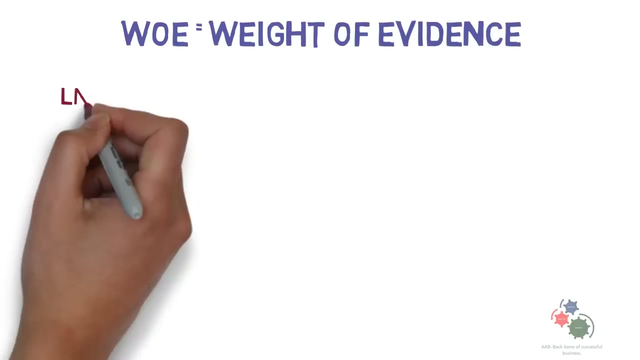 It is explained in Information Theory. It is used for Variable Selection, Grouping or Binning. Variable Predictive Strength: More is Ought, Good is the Variable We can explain WOE, Oughtage of Evidence. Log of Distribution of Good by Distribution of Bad. IV Information Value. 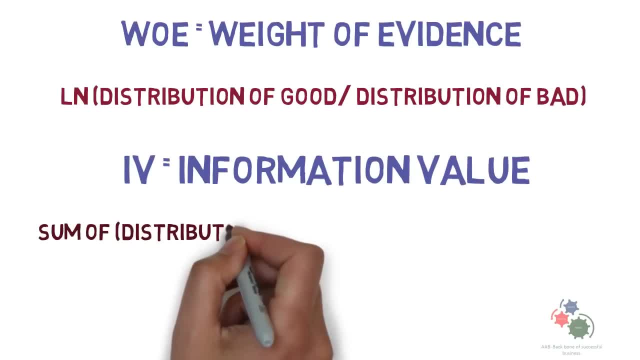 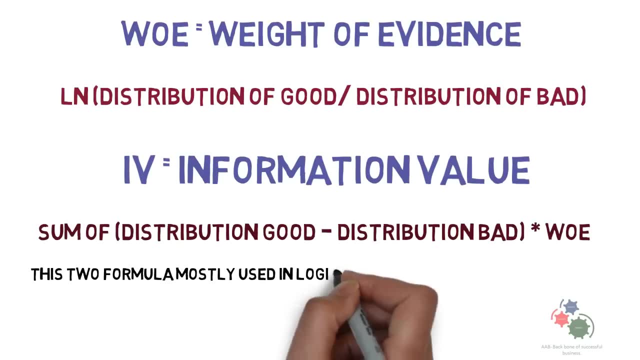 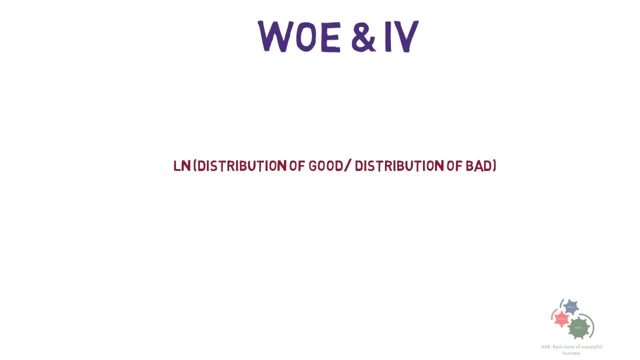 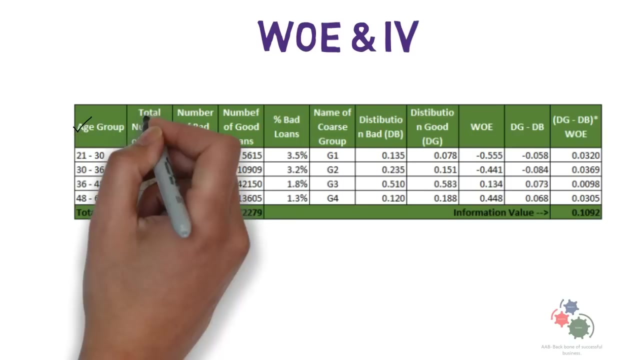 Sum of Distribution of Good minus Distribution of Bad into WOE. These two information mostly used in Logistic Regression. Let's understand the concept by below table. This is Age Group. I group the age of the customer in different groups. Total Number of Loan. 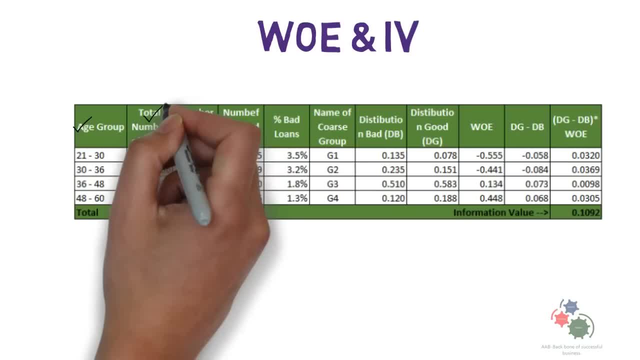 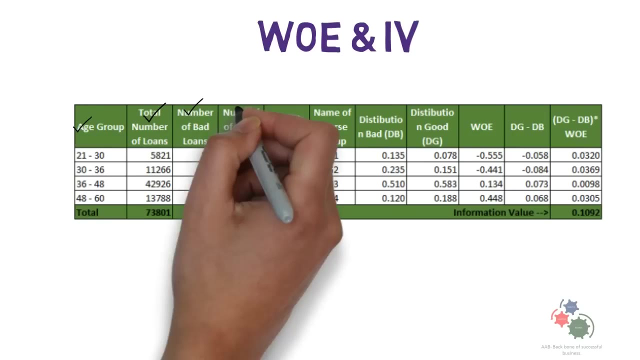 Total Number of Loan Given to different group of people in particular period. Number of Bad Loan: Out of this loan, how many are Bad Loan? Number of Good Loan: Out of this loan, how many of Good Loans? Percentage Bad Loan: Here we mention. what is the percentage of Bad Loan? 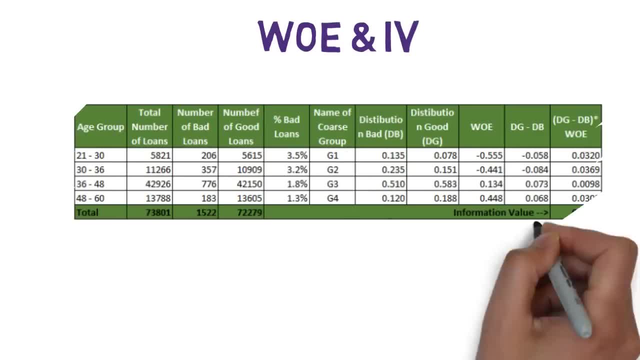 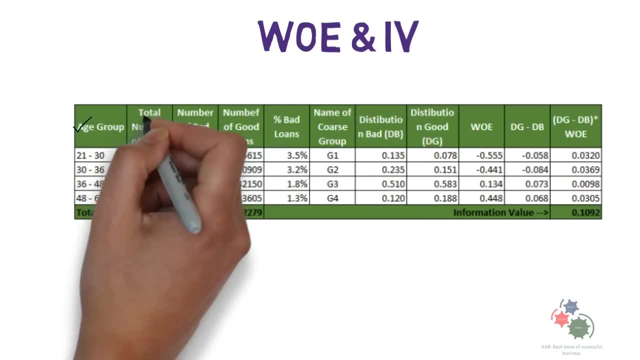 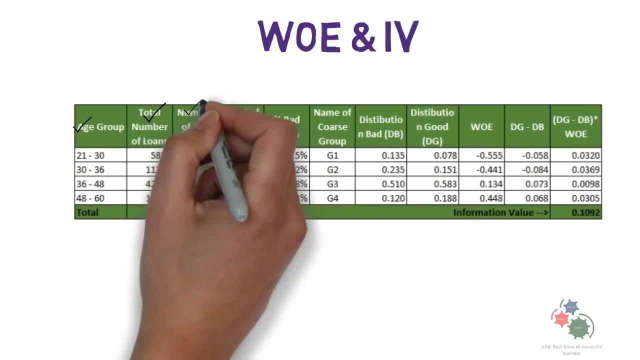 Let's understand the concept by below table. This is age group. I group the age of the customer in different groups. Total number of loan: Number of loan given to different group of people in particular. period Number of bad loan. Out of this loan, how many are bad loan? 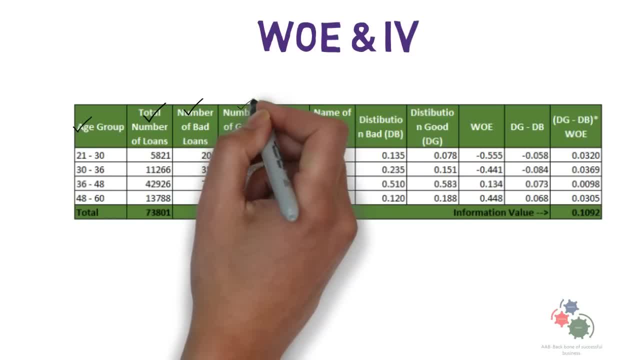 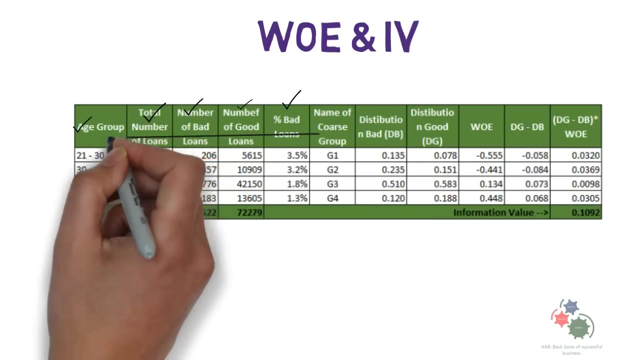 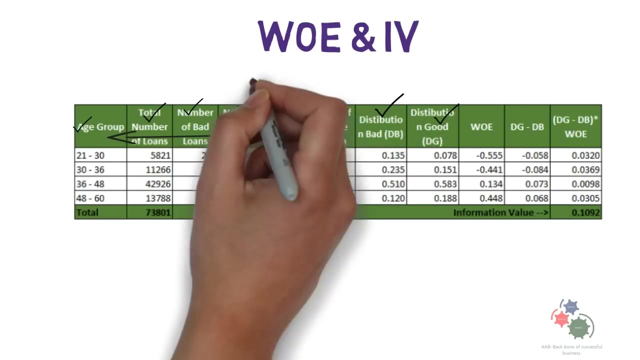 Number of good loan Out of this loan. how many of good loans? Percentage bad loan: Here we mention what is the percentage of bad loan given by the bank Name of courage group Distribution, bad Distribution, good. Now L N Logarithm of distribution of good divided by distribution. 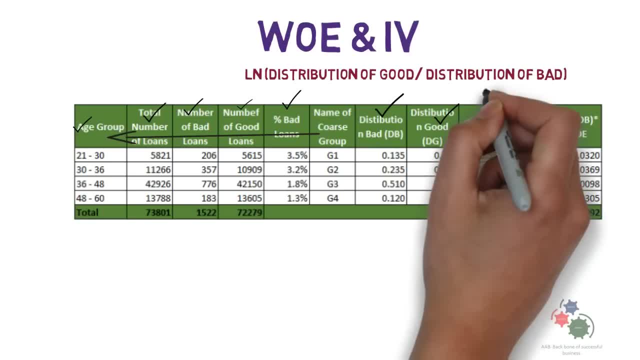 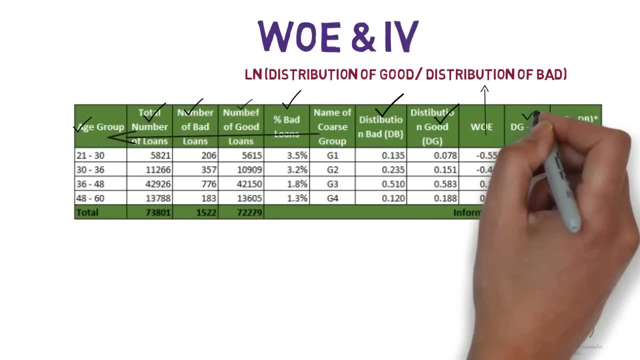 Distribution of bad. W O E. Weightage of evidence. weighted of evidence. value for every age group: Distribution good minus distribution bad. distribution good minus distribution bad. into weightage of evidence: Information value: distribution of good minus distribution of bad. 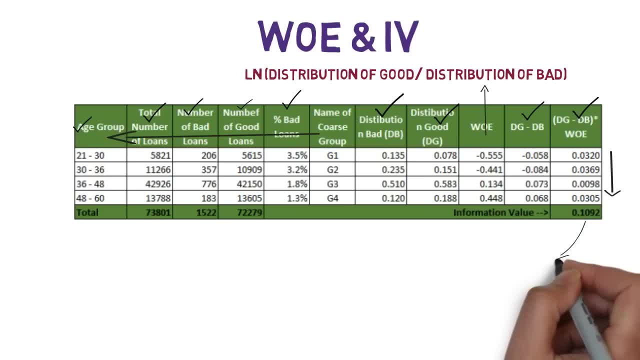 Table. We have to write a sentence like this, For example, one sentence like this: The rate of gezins is equal to Z To evaluate the H group value. to evaluate the H group value, we have to include information value in the product. 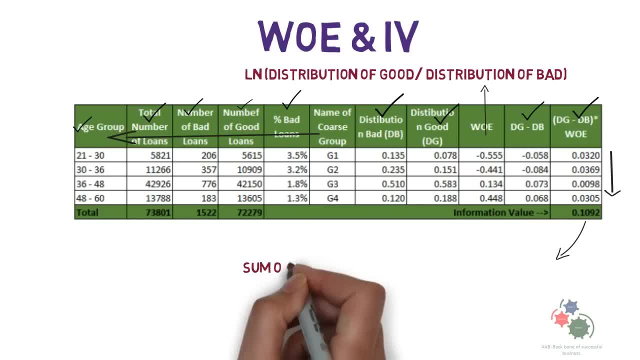 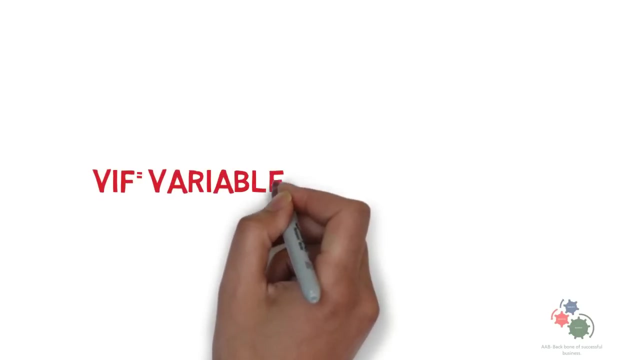 We calculate information value as sum of distribution good minus distribution bad into WOE. So information value used for variable selection, weightage of evidence used for variable grouping and binning. Our next concept is VIF- Variable Inflation Factor. A variable inflation factor is used to detect multi-collinearity in regression analysis. 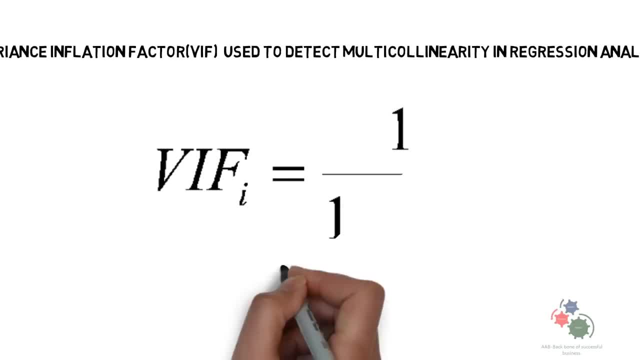 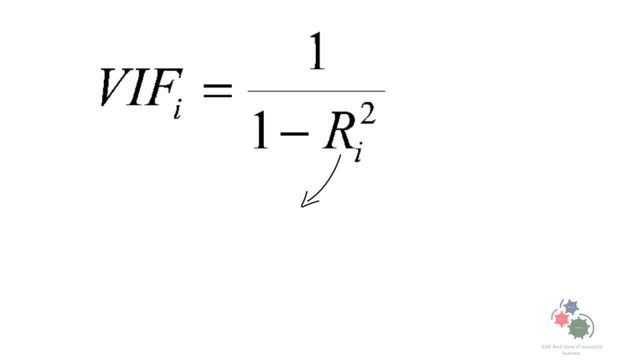 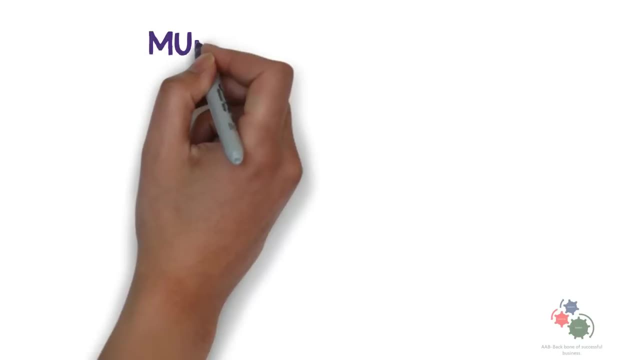 Let's understand the concept by below formula VIF: equal to 1 by 1 minus R square. Here R square equal to total variation plus unexpected variation divided by total variation. equal to explained variation divided by total variation. Let's understand the concept by multiple regression. 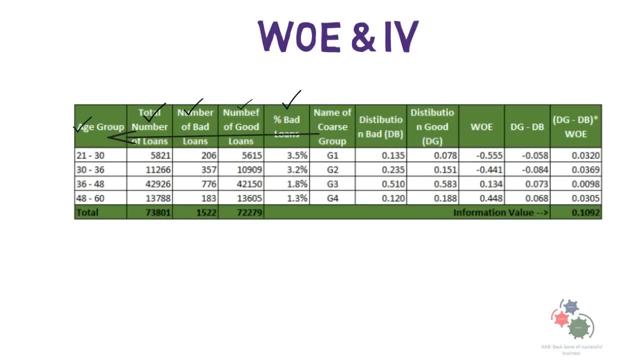 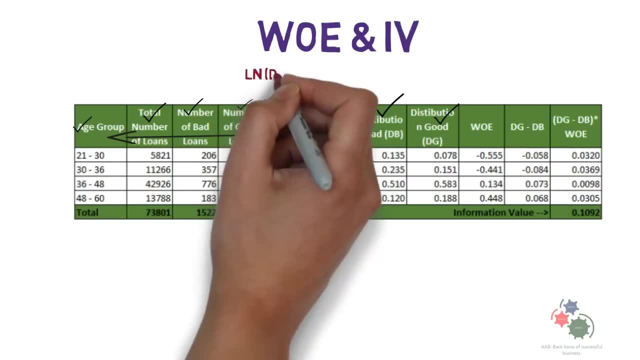 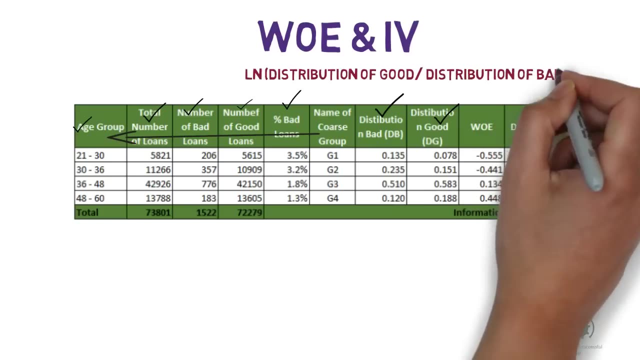 given to people in particular, period given by the bank name of courage. group distribution: bad distribution, good. now ln logarithm of distribution of good divided by distribution of bad. woe weightage of evidence. weightage of evidence: value for every age. group distribution: good minus distribution: bad distribution, good. 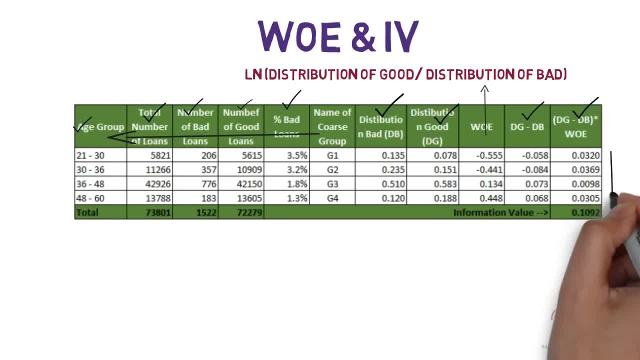 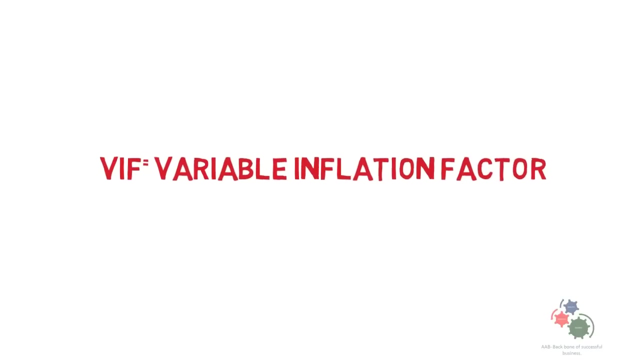 minus distribution bad into weightage of evidence. information value: we calculate information value as sum of distribution good minus distribution bad into woe. so information value used for variable selection, weightage of evidence used for variable grouping and winning. our next concept is vif- variable inflation factor a. 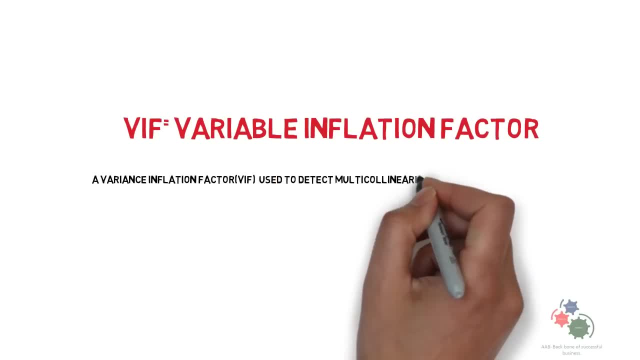 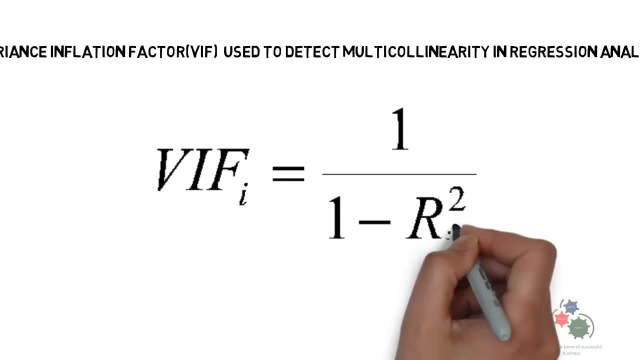 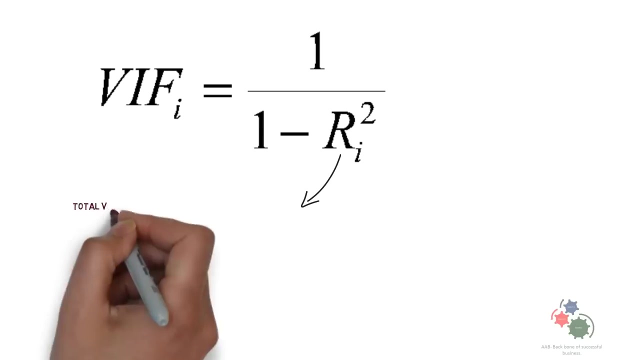 variable inflation factor is used to detect multi-collinearity in regression analysis. let's understand it. the concept by below formula vif equal to 1 by 1 minus r square. here r square equal to total variation plus unexpected variation. divided by total variation, equal to explained. 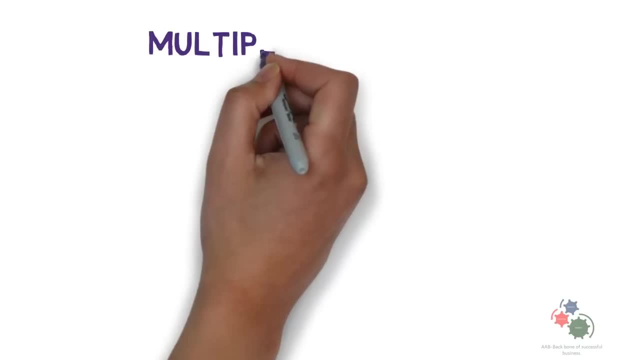 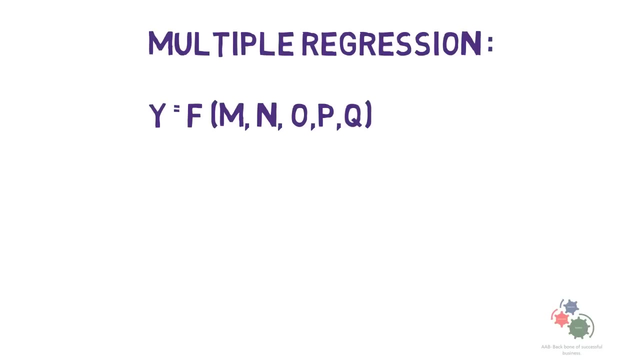 variation divided by total variation. Let's understand the concept by multiple regression. y is equal to function of M N O P Q. here focus on M N O P Q. they are independent variable. Pick up one variable and run linear regression with other variables by running: 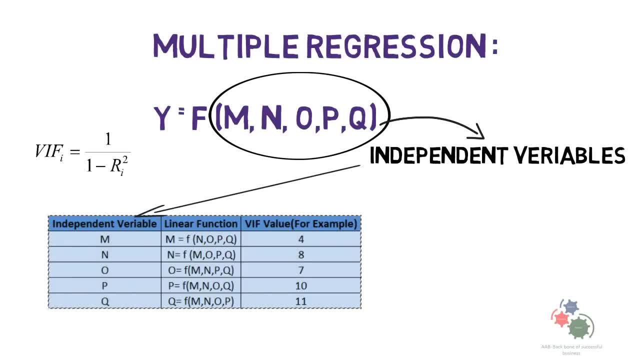 linear regression. by running linear regression, by considering one variable as dependent variable, we will get r square of that variable. from r square we can able to calculate vif of that variable. say, for example, in this table, vif value of m is 4, n is 8, o is 7, p is 10, q is 11. range of vif value: